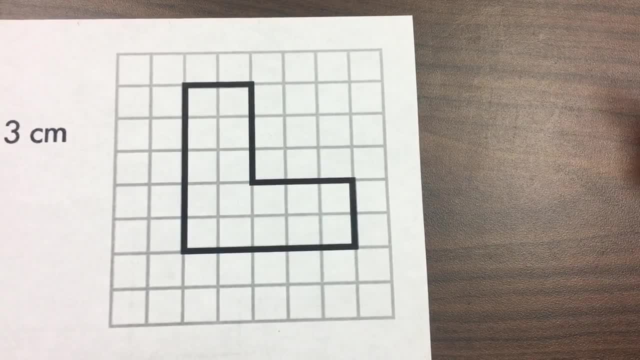 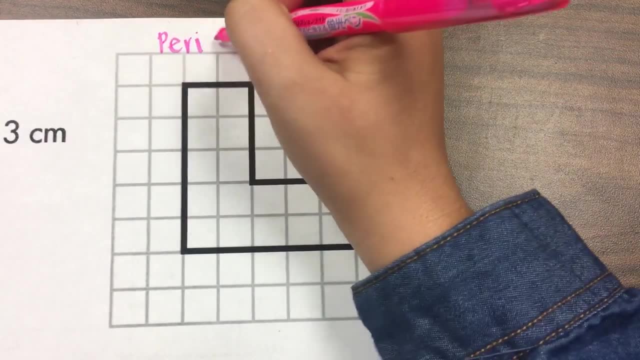 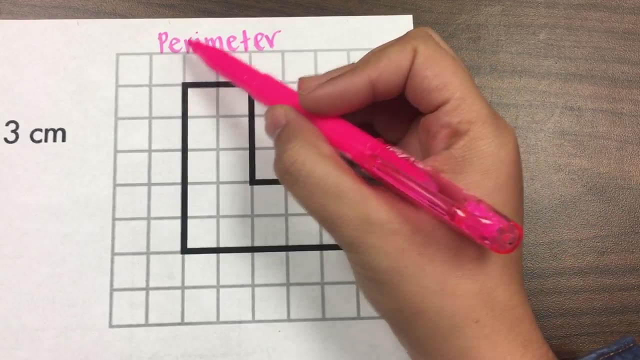 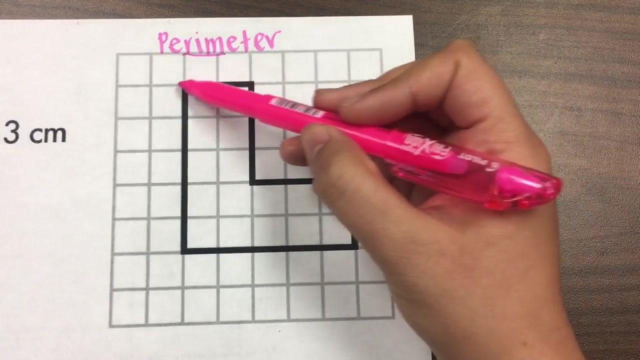 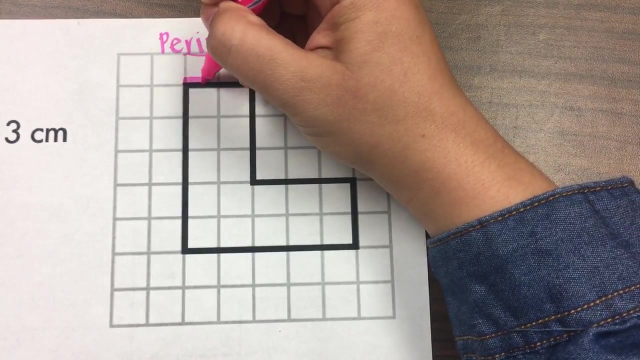 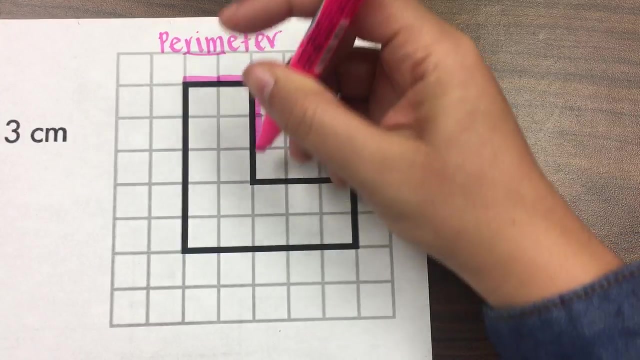 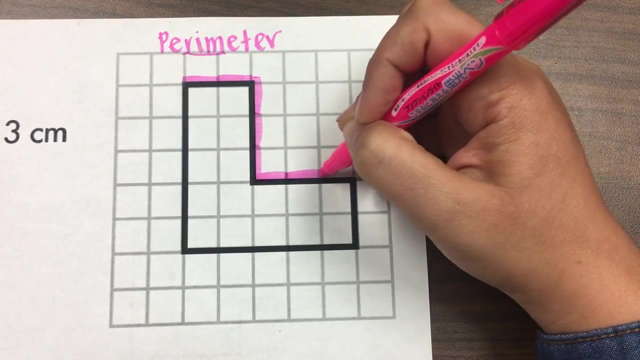 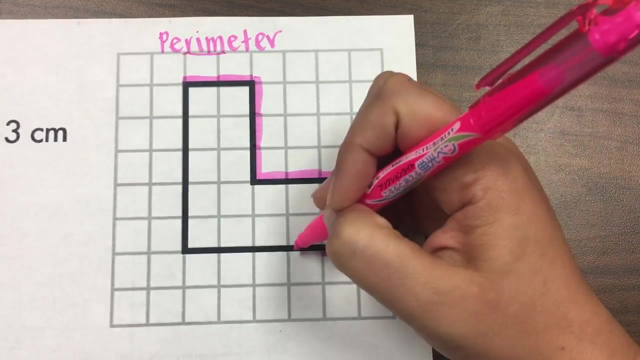 So we're going to review the perimeter. So remember that the perimeter is the outside. So if you look at the word perimeter, you can see the word rim, which is the outside of the figure, Like the outside. So this is going to be 1,, 2,, 3,, 4,, 5,, 6,, 7,, 8,, 9,, 10,, 11,, 12,, 13,, 14,, 15,, 16,, 17,, 18,, 19, 20.. 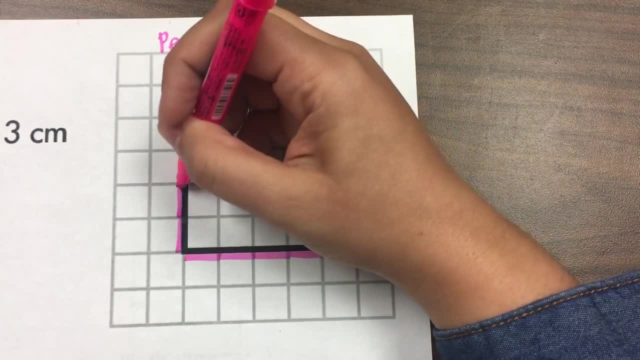 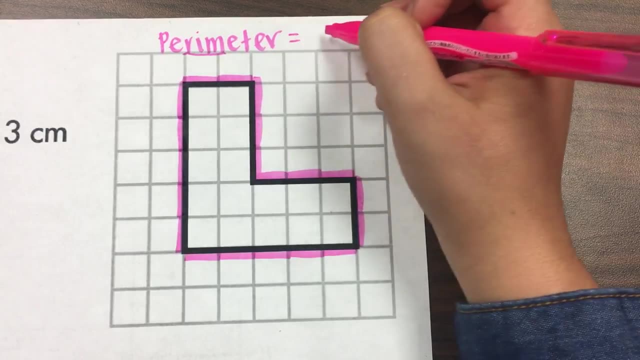 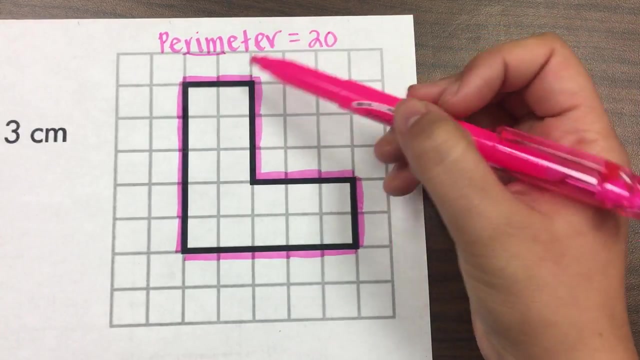 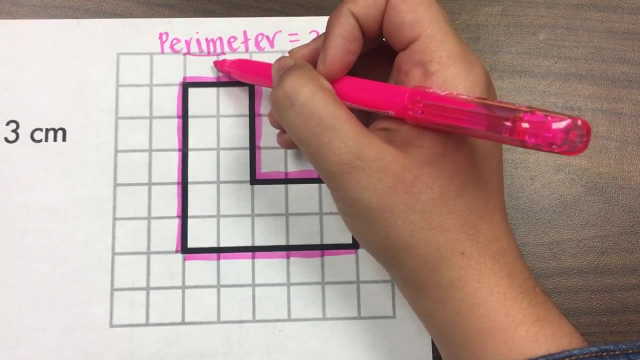 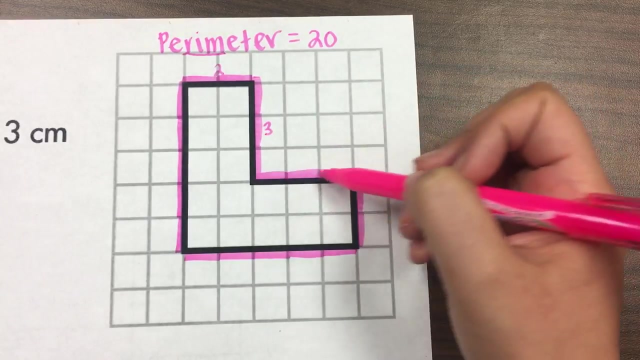 16,, 17,, 18,, 19,, 20.. So my perimeter would be equal to 20.. Now you can also count each side. So for example: here I have 2.. Here I have 3.. Here I have 3 again. 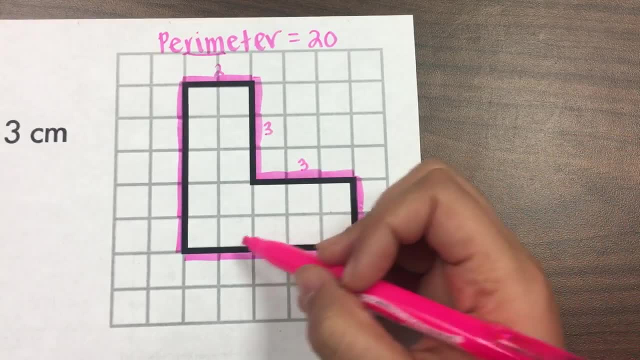 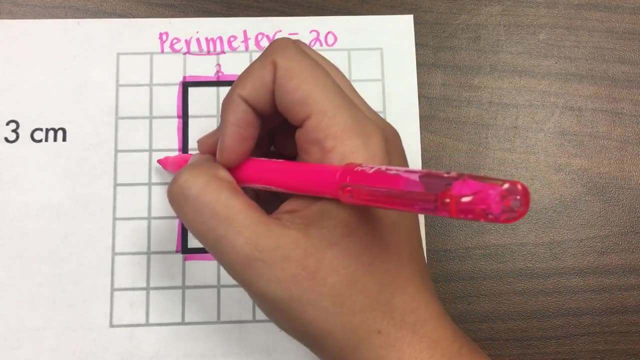 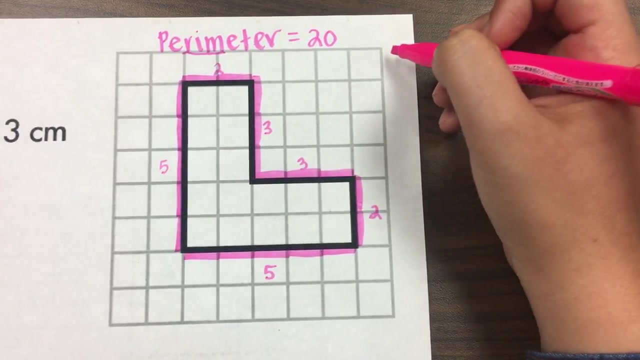 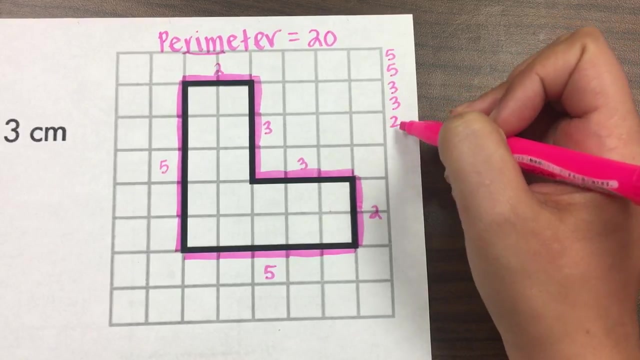 Here I have 2.. Here I have 5. And here I have 5.. And once you have all your numbers, you can also add them. So 5 plus 5 plus 3 plus 3 plus 2 plus 2.. 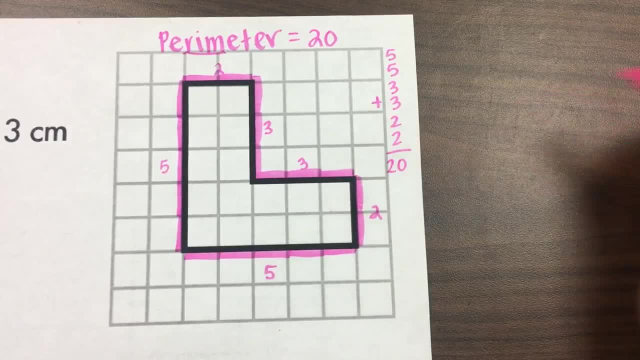 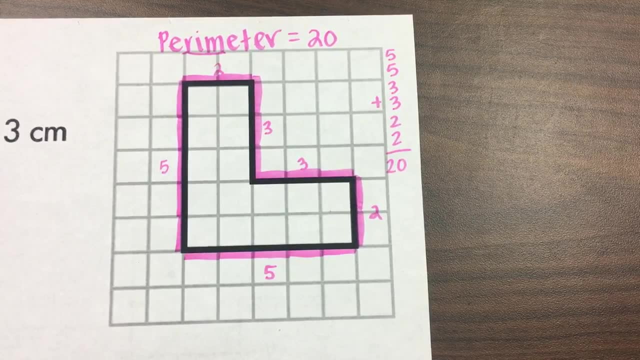 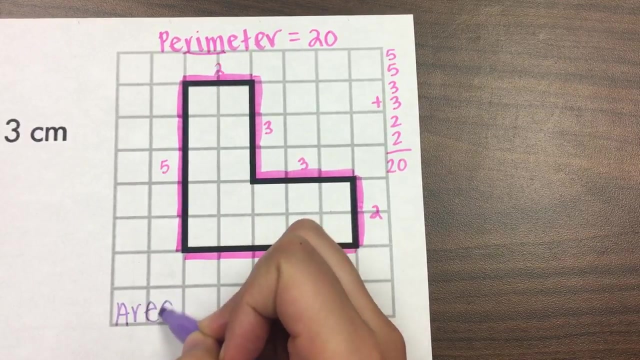 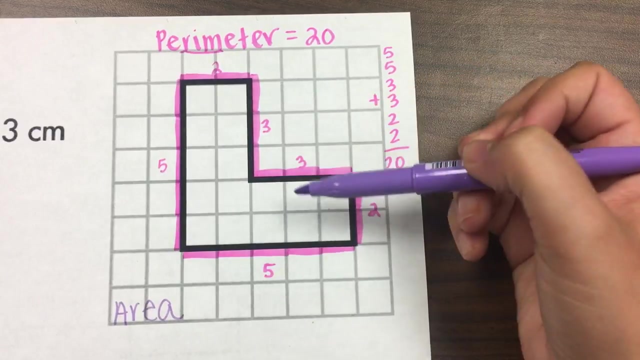 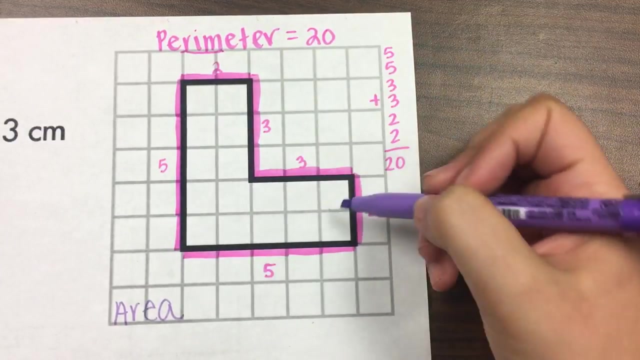 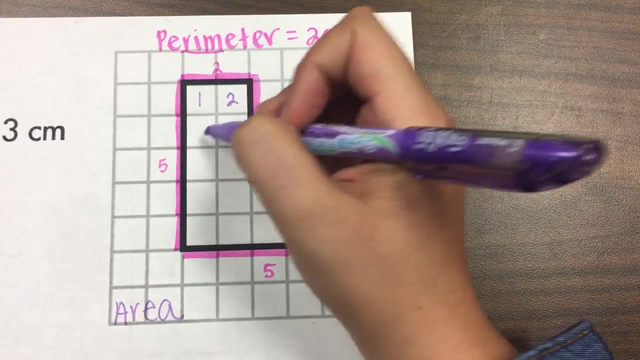 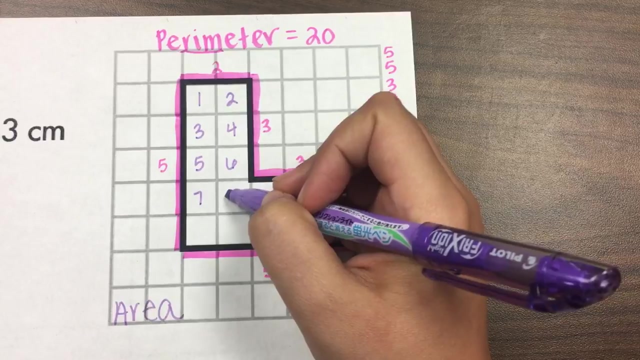 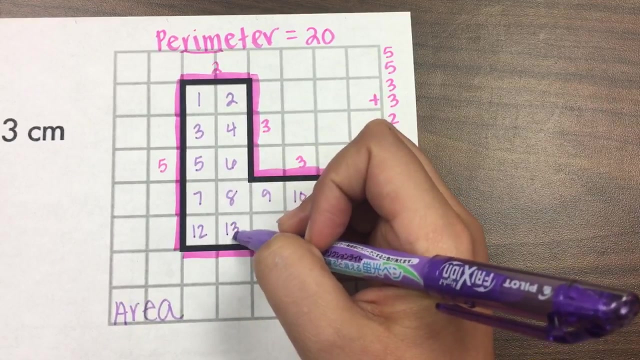 Should add up to 20 also. Okay. Now we're going to be talking about area. Okay, And area is the inside of your irregular figure, So you can Count all the cubes that are inside, For example, 1, 2,, 3,, 4,, 5,, 6,, 7,, 8,, 9,, 10,, 11,, 12,, 13,, 14,, 15, 16.. 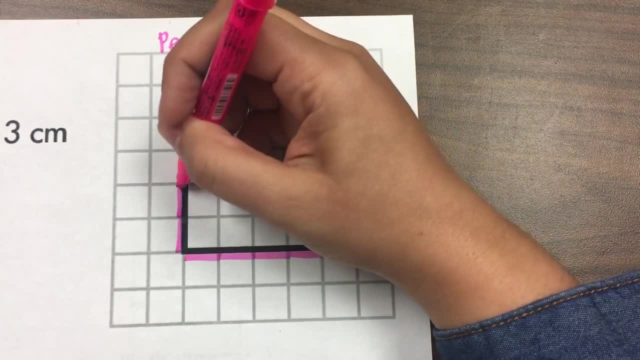 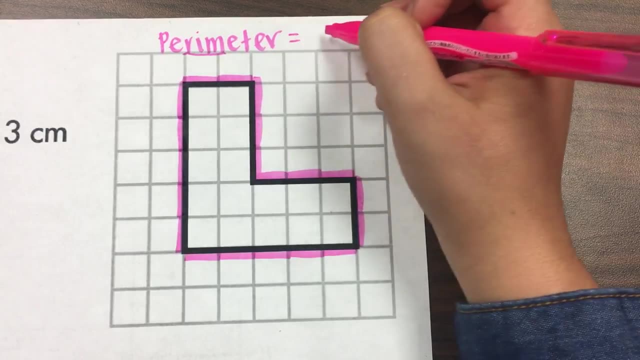 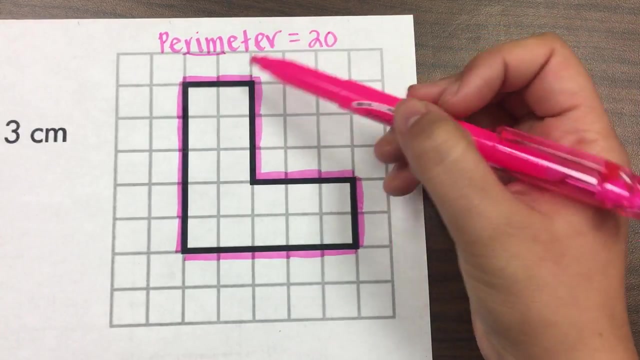 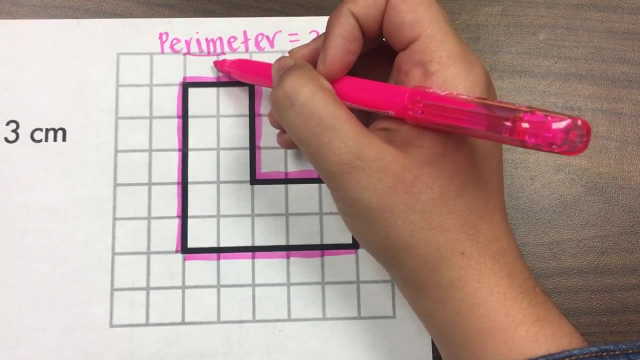 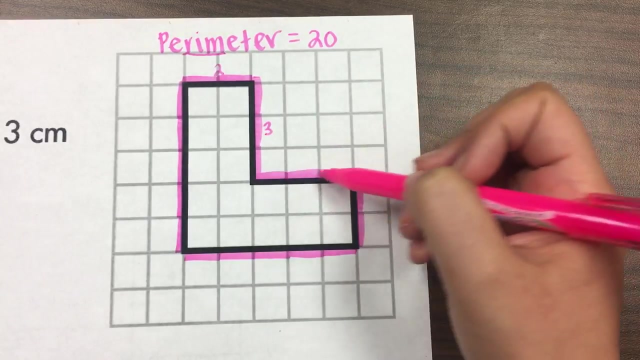 16,, 17,, 18,, 19,, 20.. So my perimeter would be equal to 20.. Now you can also count each side. So for example: here I have 2.. Here I have 3.. Here I have 3 again. 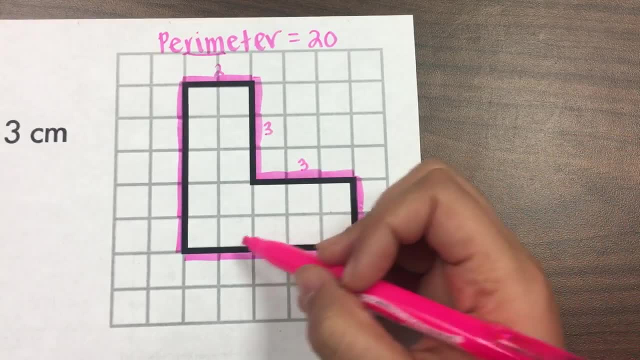 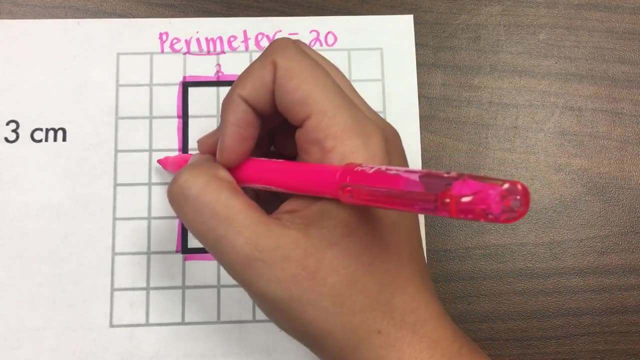 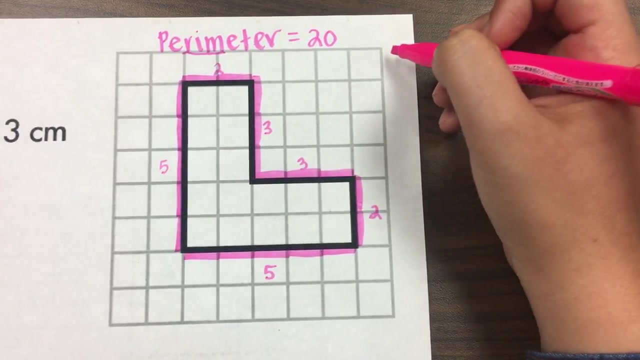 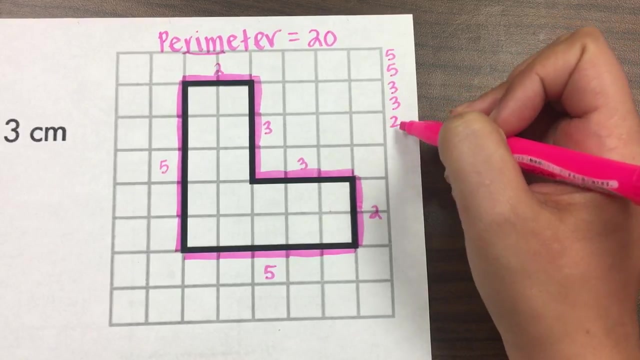 Here I have 2.. Here I have 5. And here I have 5.. And once you have all your numbers, you can also add them. So 5 plus 5 plus 3 plus 3 plus 2 plus 2.. 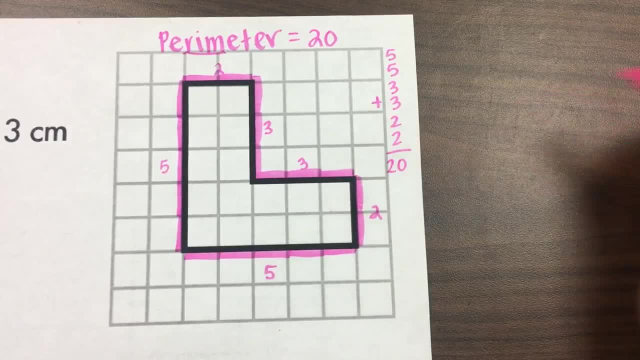 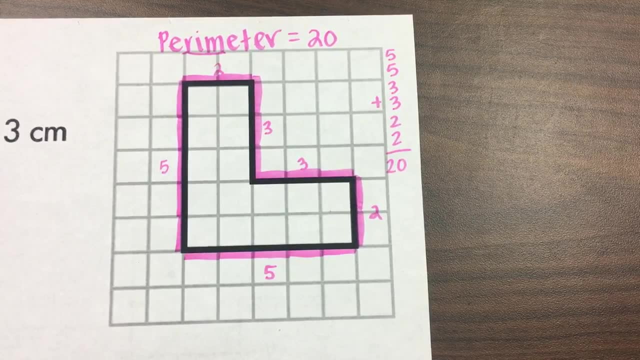 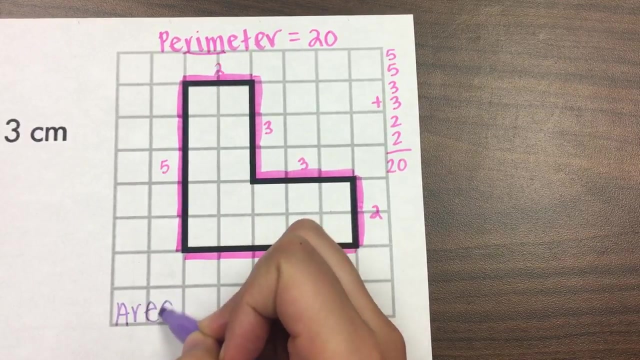 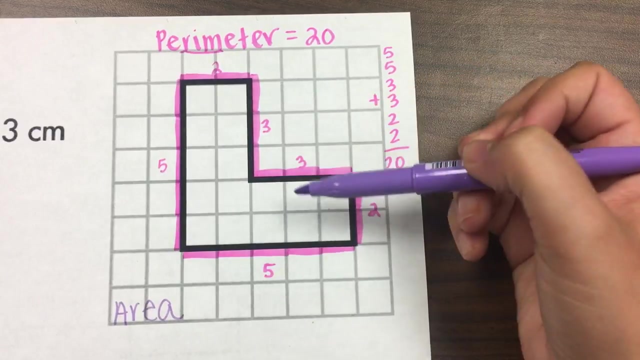 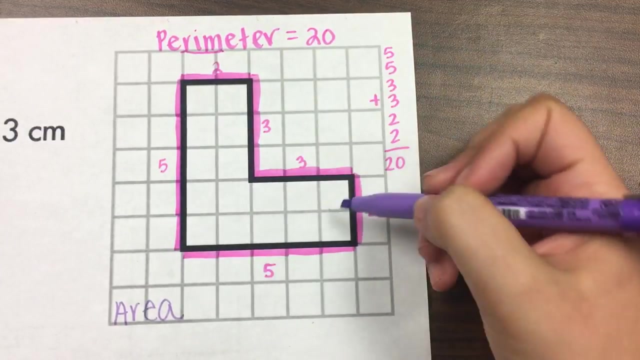 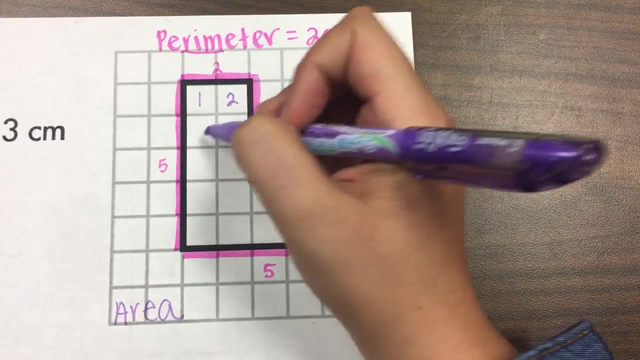 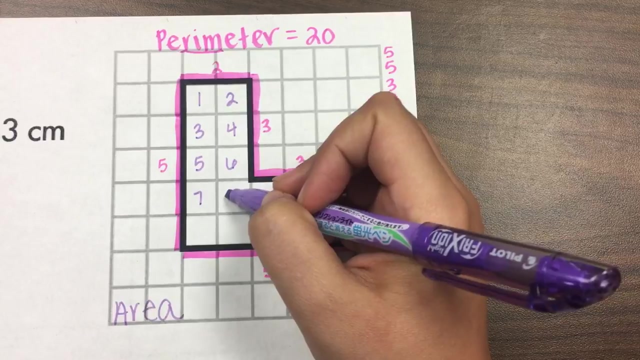 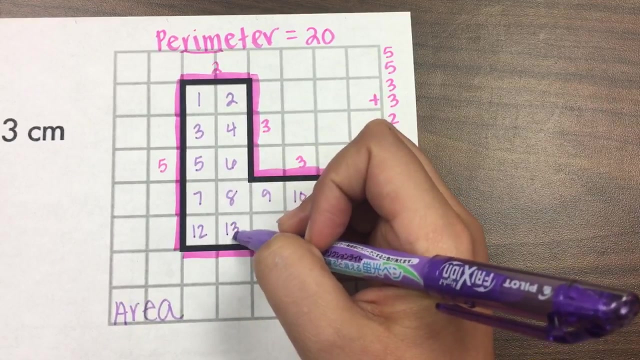 Should add up to 20 also. Okay. Now we're going to be talking about area. Okay, And area is the inside of your irregular figure, So you can Count all the cubes that are inside, For example, 1, 2,, 3,, 4,, 5,, 6,, 7,, 8,, 9,, 10,, 11,, 12,, 13,, 14,, 15, 16.. 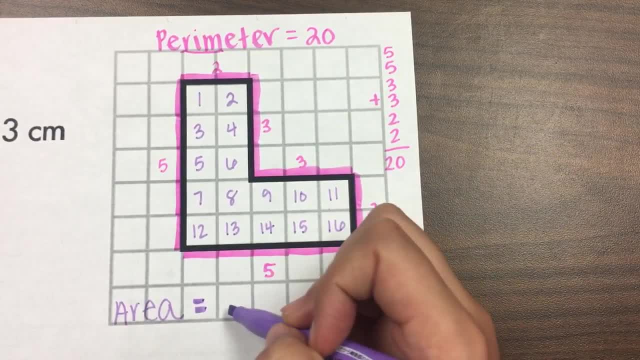 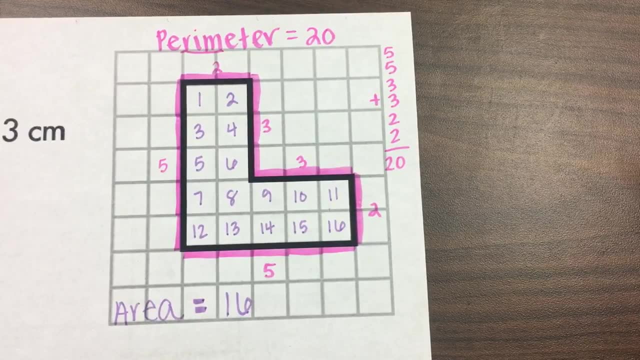 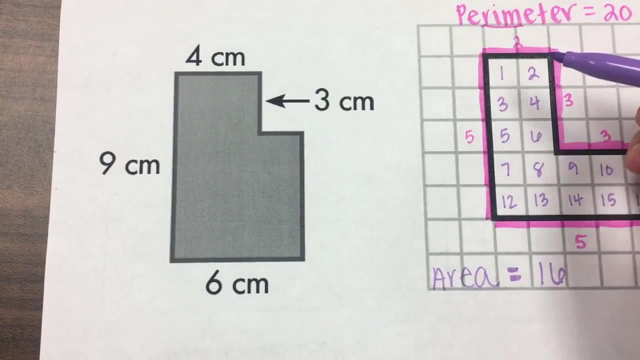 So the area Would be equal to 16 units. Okay, And that's how you would find perimeter and area. Now let's try an example where they don't give you all the squares that are on the inside. So first let's start with perimeter again. 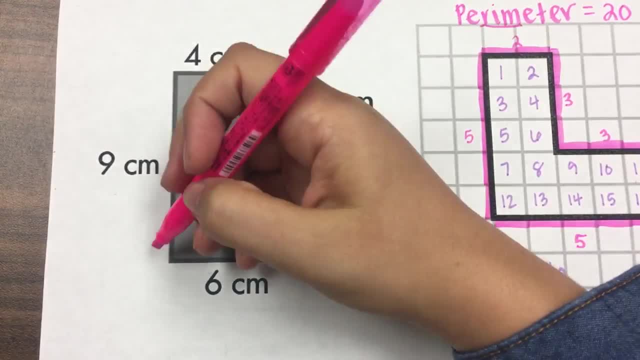 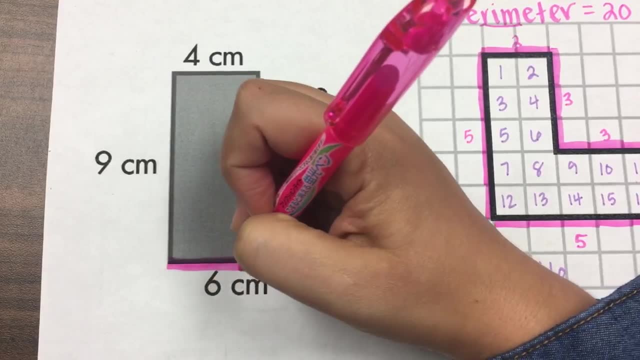 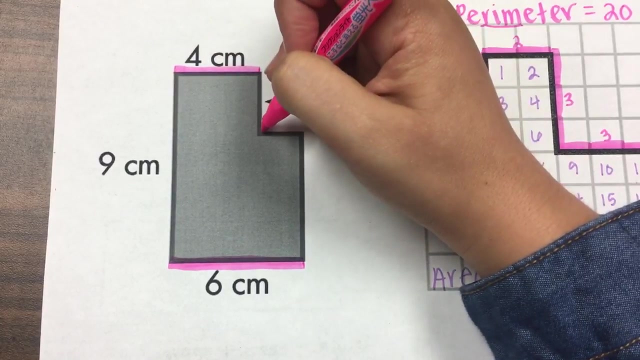 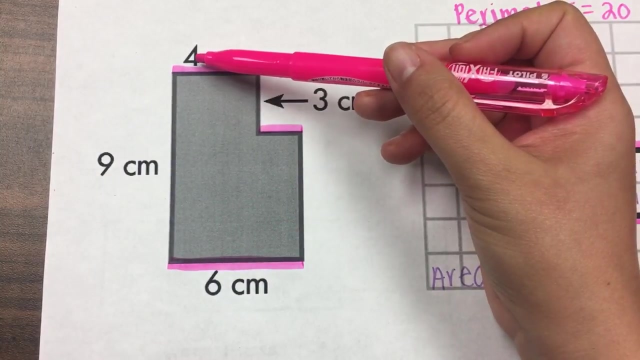 And if we know that this section Is equal to 6. Then the opposite section should also be equal to 6.. So this plus this should equal to 6.. So if I have 4, I need 2 more, So the 2 would go here. 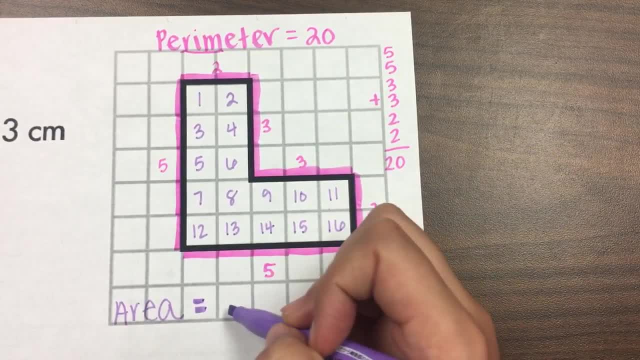 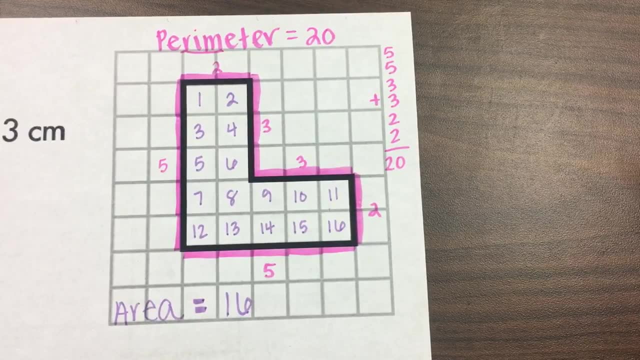 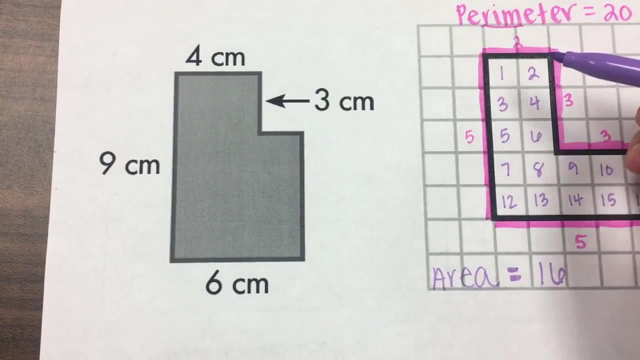 So the area Would be equal to 16 units. Okay, And that's how you would find perimeter and area. Now let's try an example where they don't give you all the squares that are on the inside. So first let's start with perimeter again. 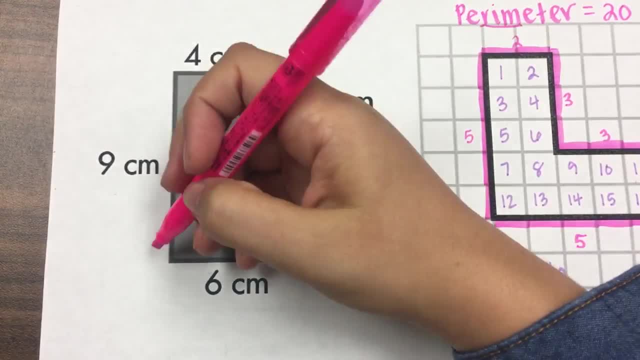 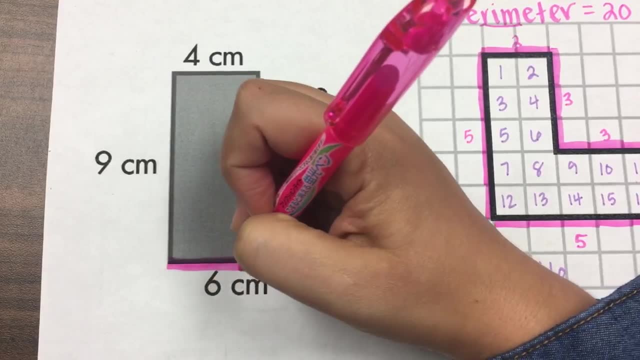 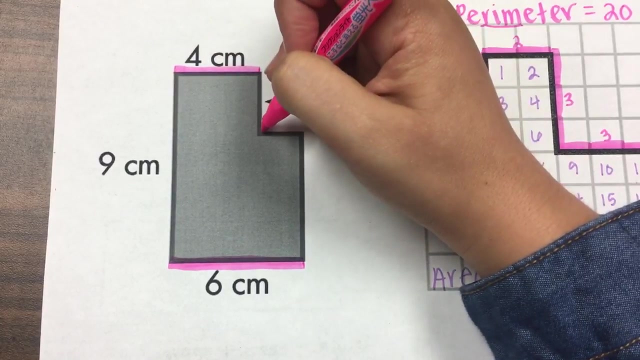 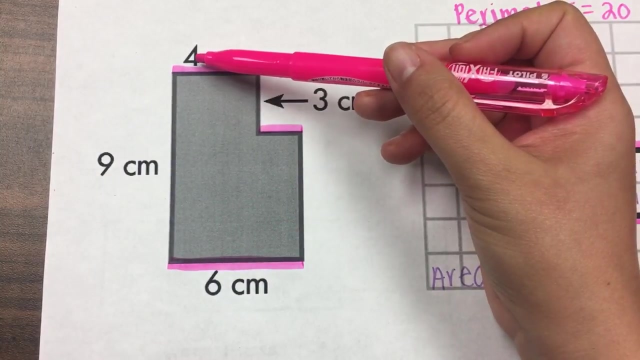 And if we know that this section Is equal to 6. Then the opposite section should also be equal to 6.. So this plus this should equal to 6.. So if I have 4, I need 2 more, So the 2 would go here. 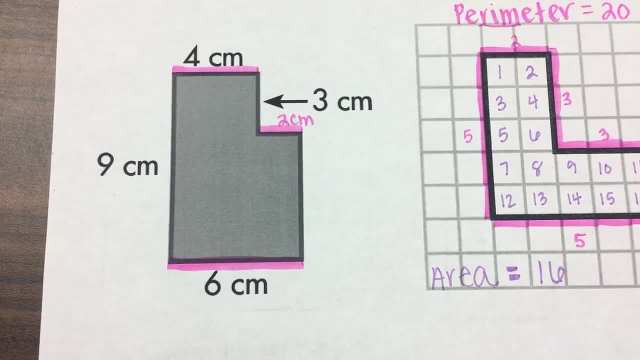 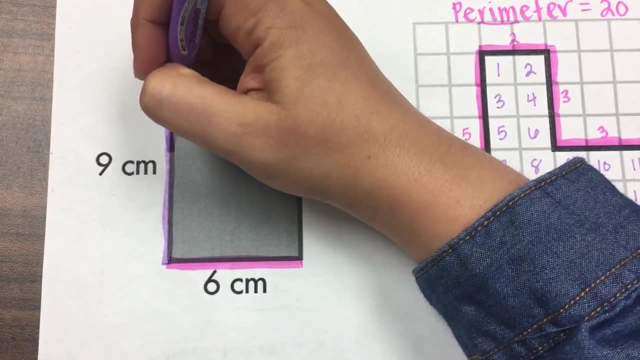 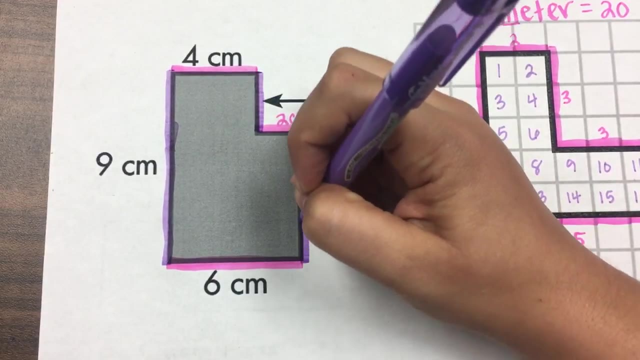 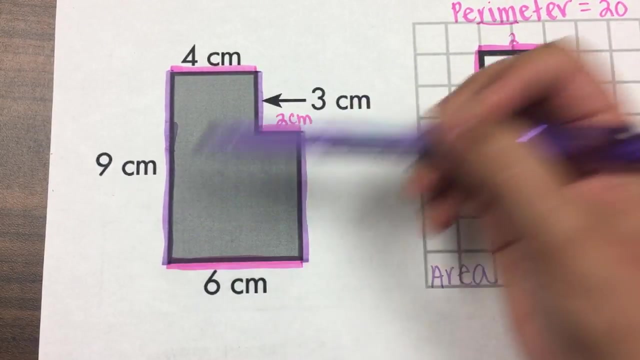 Okay, Then On this side, I know that this side is equal to 9.. Which means that this 3 plus this has to equal 9 as well. So if I have 9 as my total, Then 3 plus 6 more. 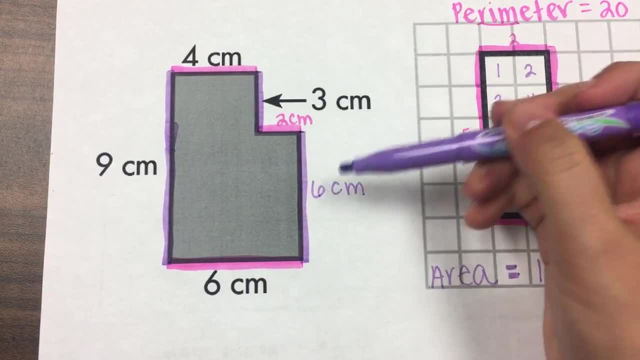 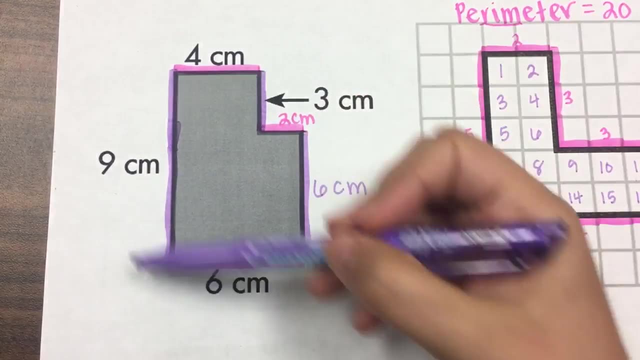 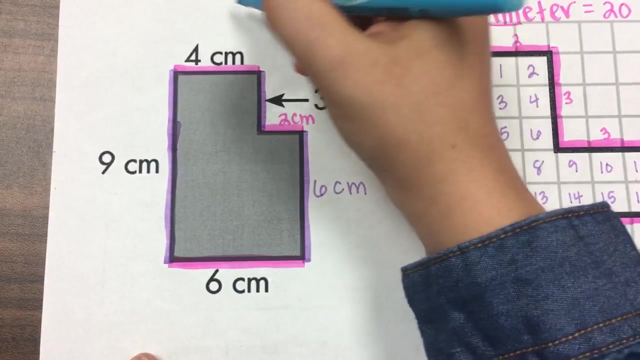 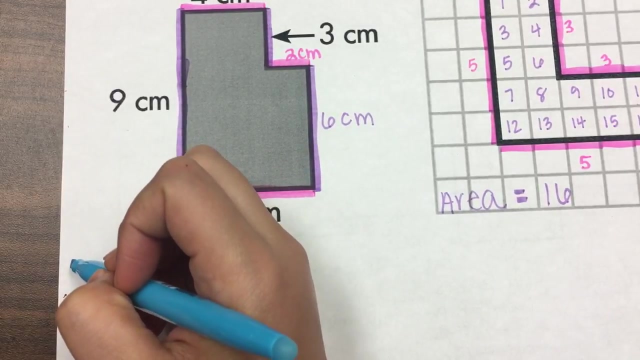 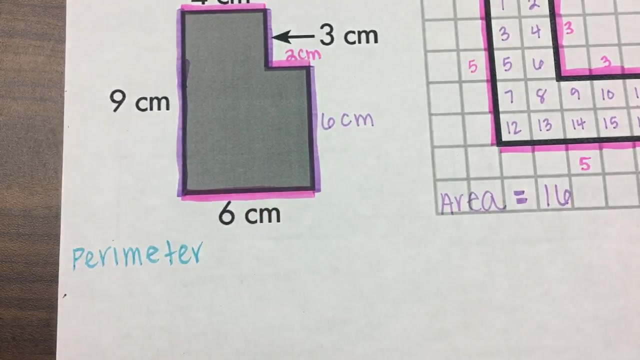 Would give me 9.. 6 plus 3 is 9.. Okay, Now that I have all of my numbers, I'm able to find the perimeter. Let's do it down here Now. remember that perimeter is All of the numbers on the outside. 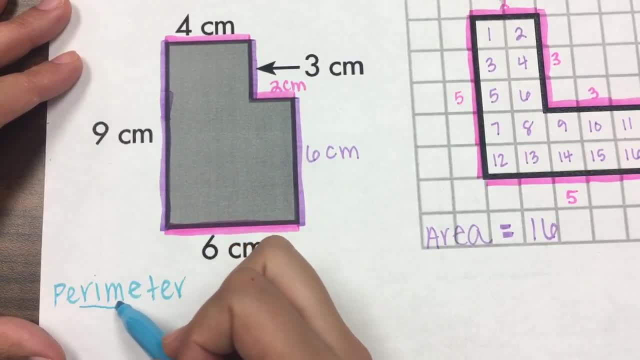 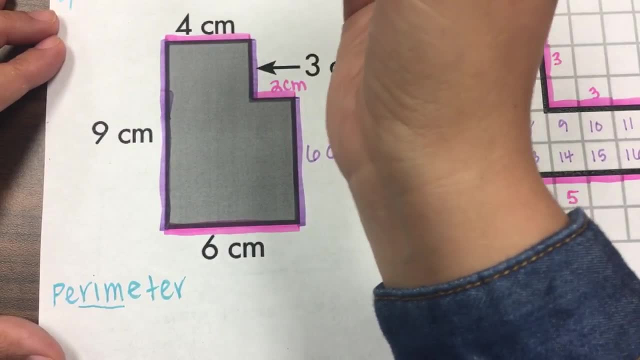 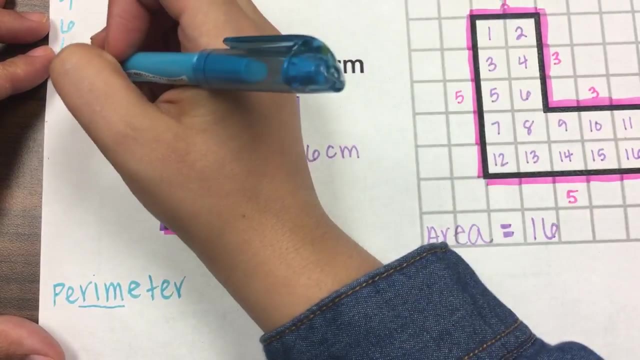 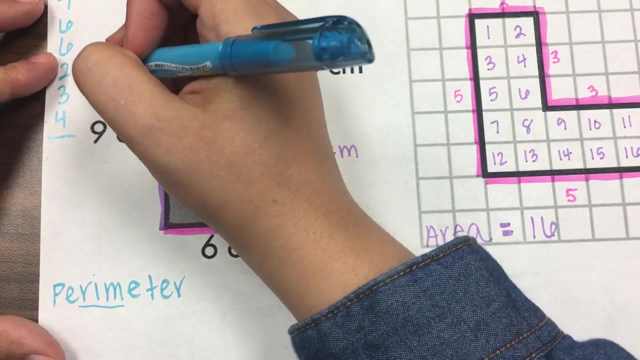 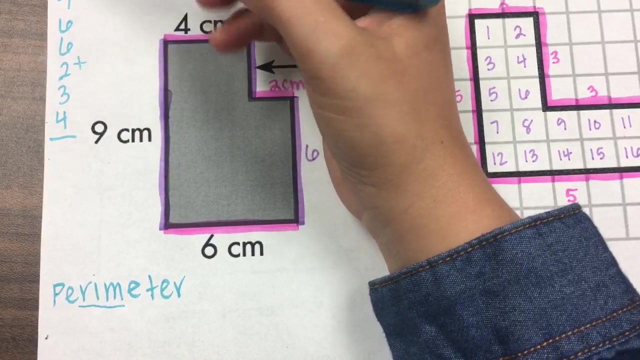 The rim. Okay, Think of the word Rim. Okay, So we need to add 9. Plus 6. Plus 6. Plus 2. Plus 3. Plus 4.. Okay, Okay, So All right. 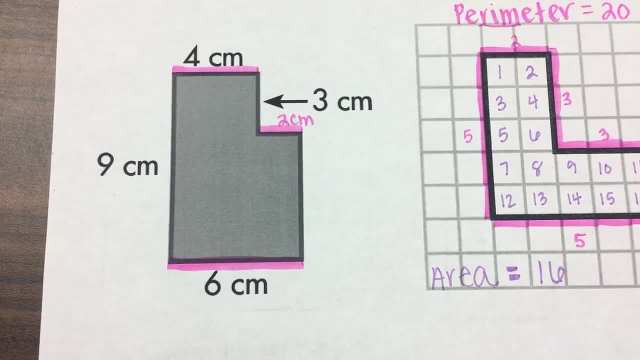 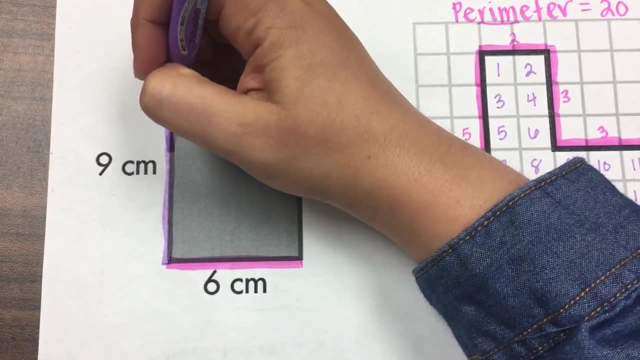 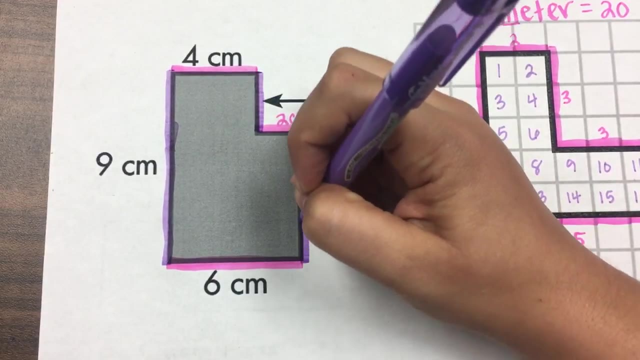 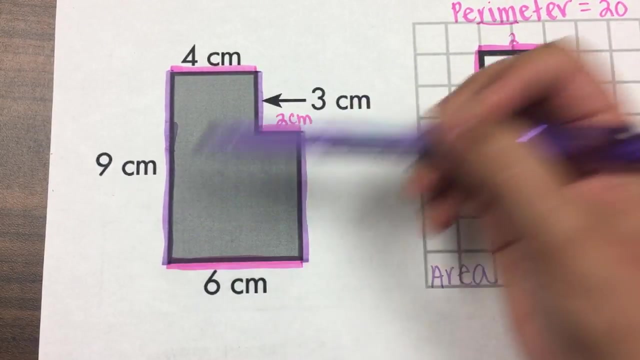 Okay, Then On this side, I know that this side is equal to 9.. Which means that this 3 plus this has to equal 9 as well. So if I have 9 as my total, Then 3 plus 6 more. 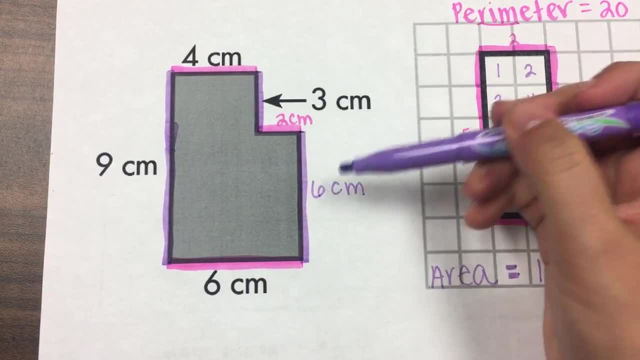 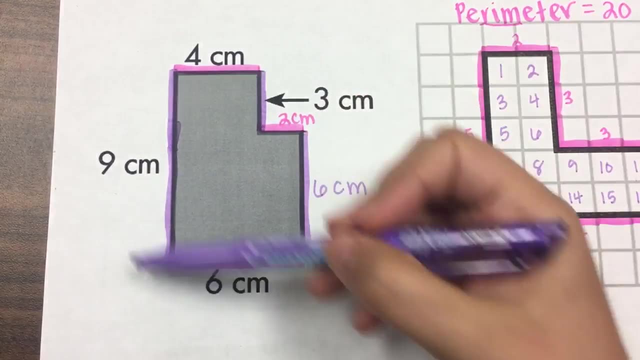 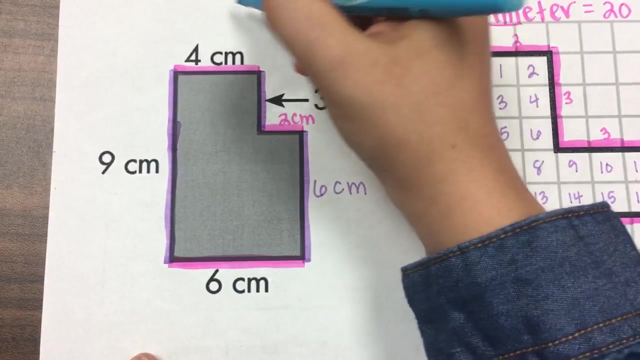 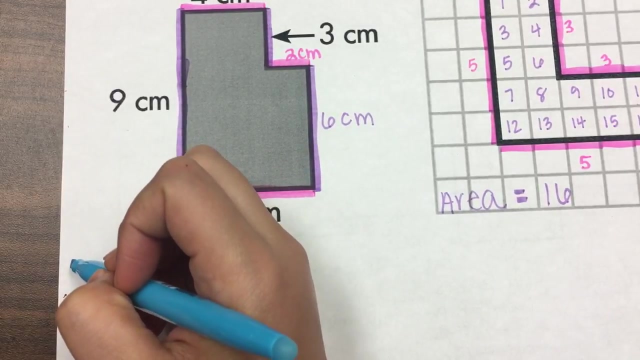 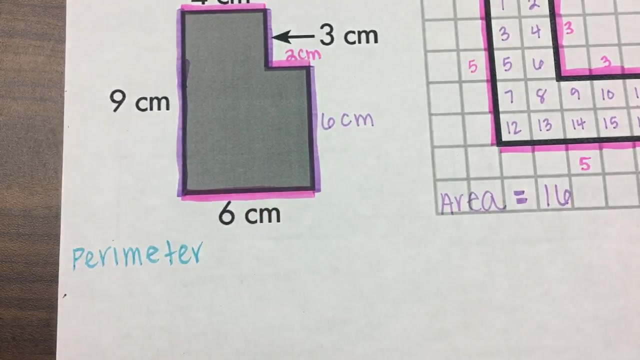 Would give me 9.. 6 plus 3 is 9.. Okay, Now that I have all of my numbers, I'm able to find the perimeter. Let's do it down here Now. remember that perimeter is All of the numbers on the outside. 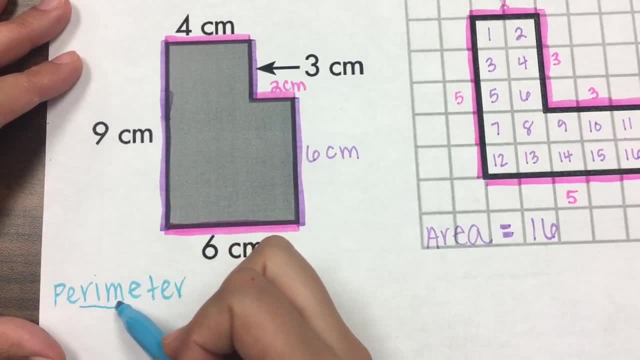 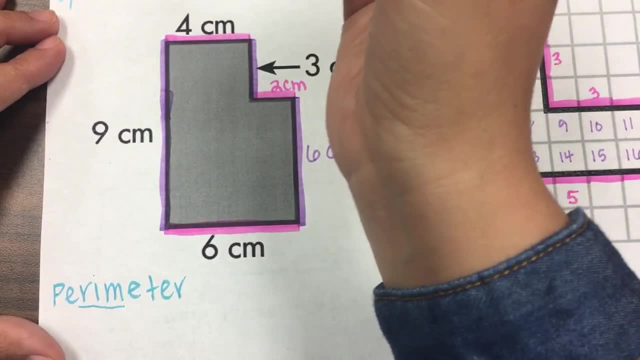 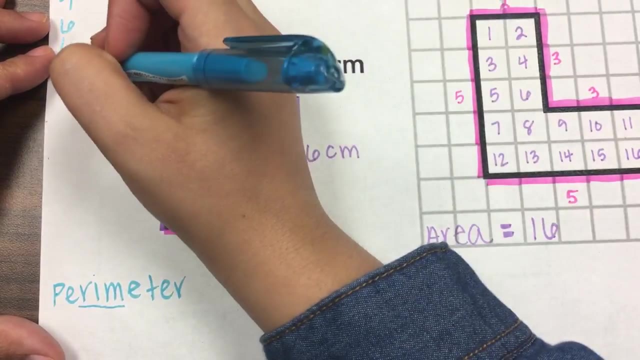 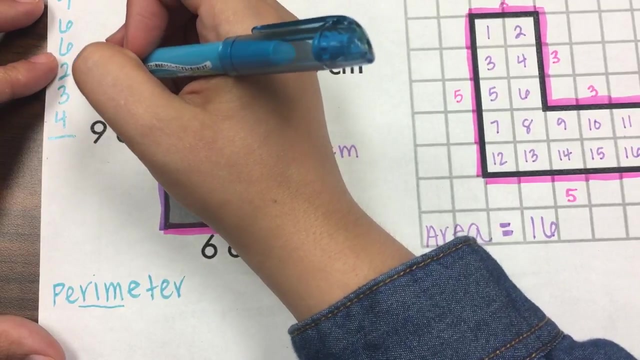 The rim. Okay, Think of the word Rim. Okay, So we need to add 9. Plus 6. Plus 6. Plus 2. Plus 3. Plus 4.. Okay, Okay, So I have 3.. 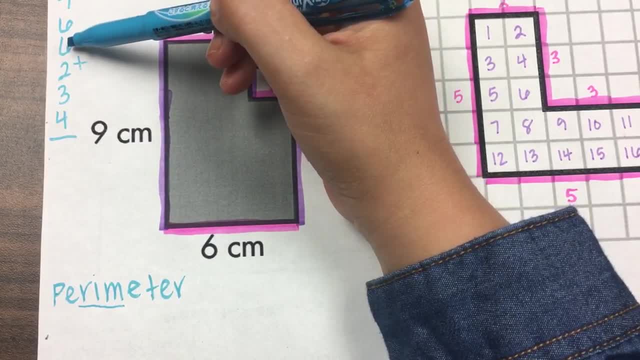 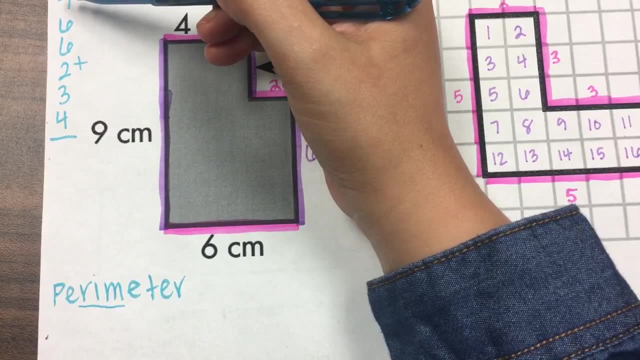 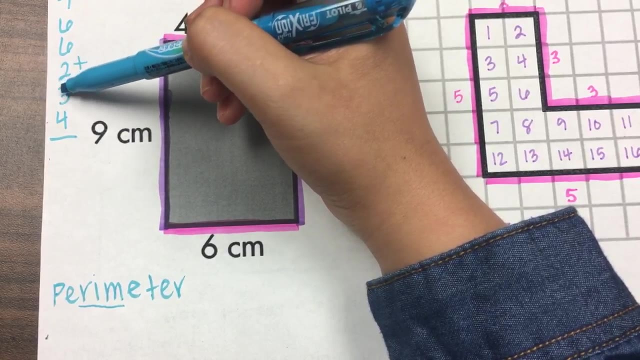 6 plus 1.. Alright, So 6 plus 4 is 10.. Plus 9 is 19.. 18,, 20,, 21,, 22,, 23,, 24.. Plus 6 more is 30.. 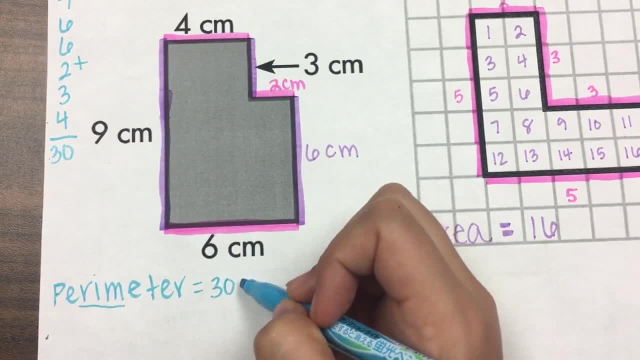 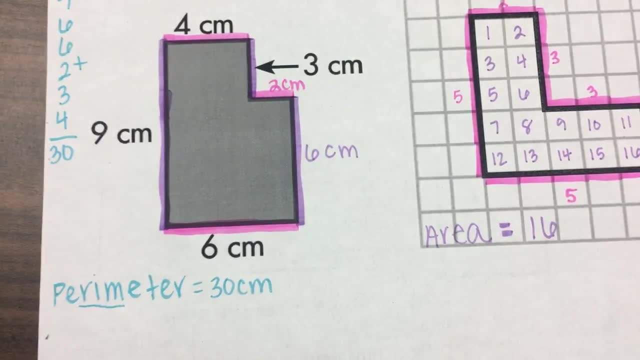 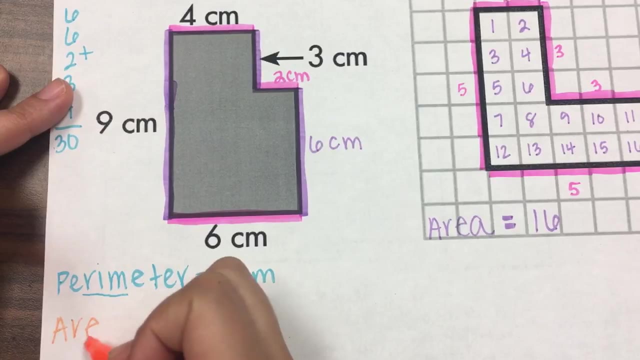 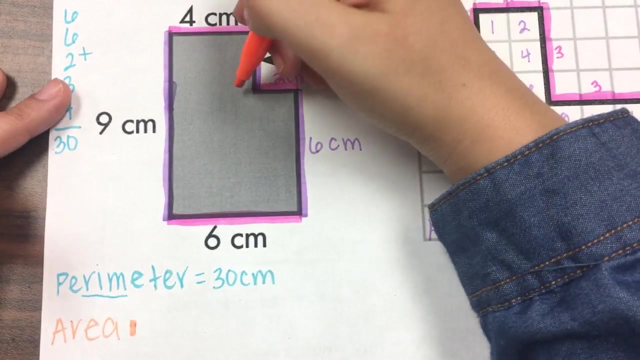 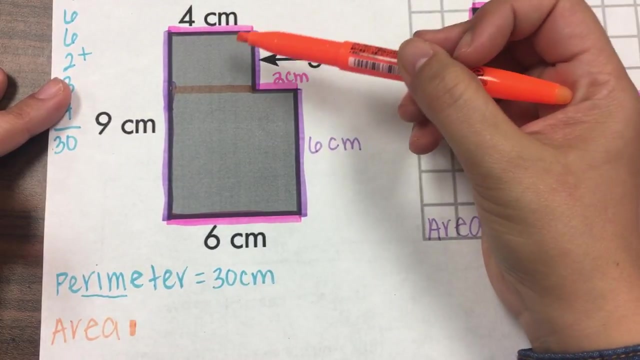 So the perimeter would equal to 30 centimeters. okay, now to find area. Okay, To find area. we're gonna have to cut this into two pieces. so If I cut this in half Now, I have two regular shapes. I have a small rectangle up here and 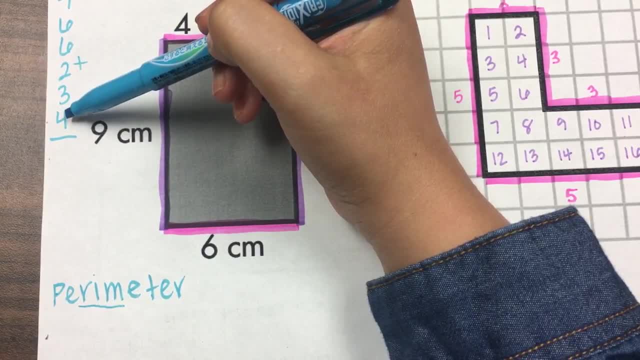 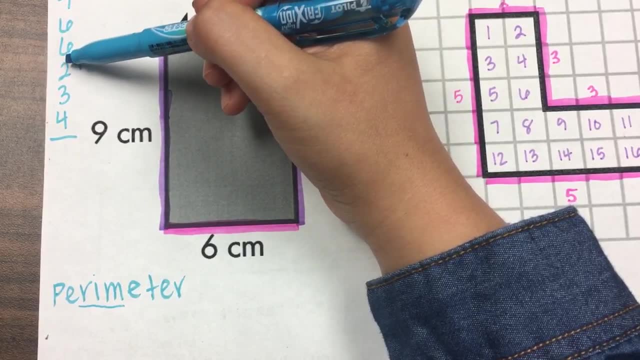 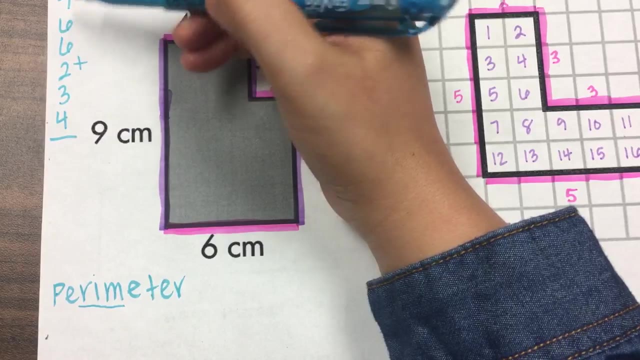 So 6 plus 4 is 10., Plus 9. Is 19., 18., 20., 21., 22., 23., 24. Plus 6 more is 30. So the perimeter would equal 2.. 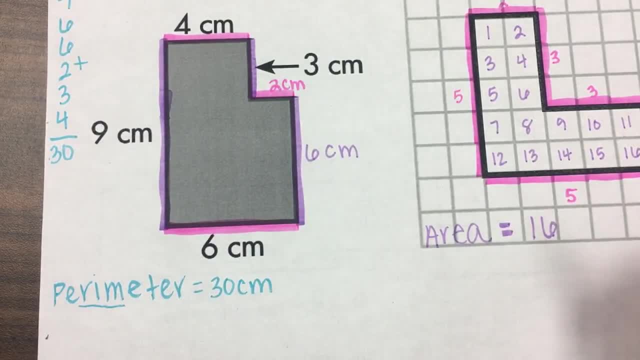 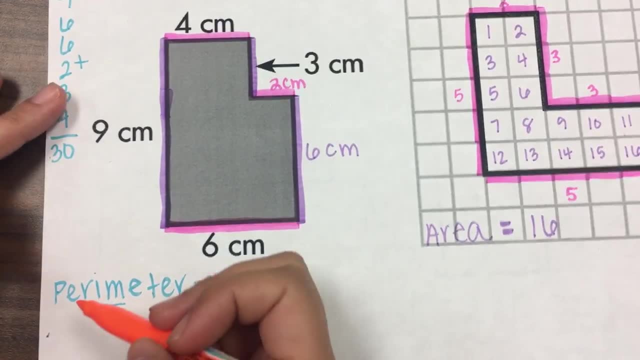 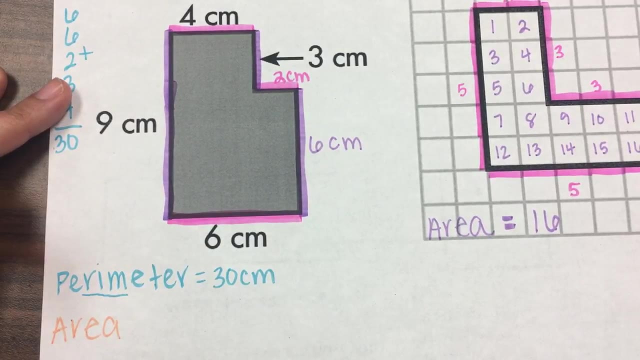 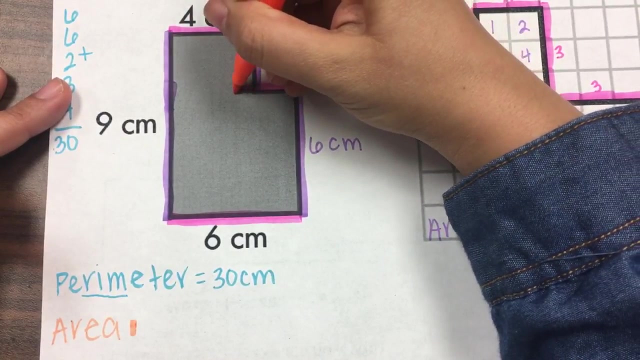 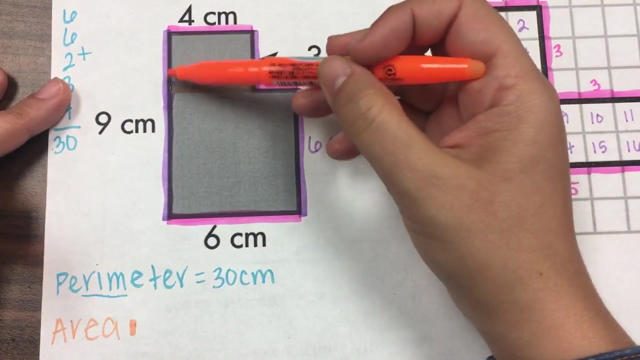 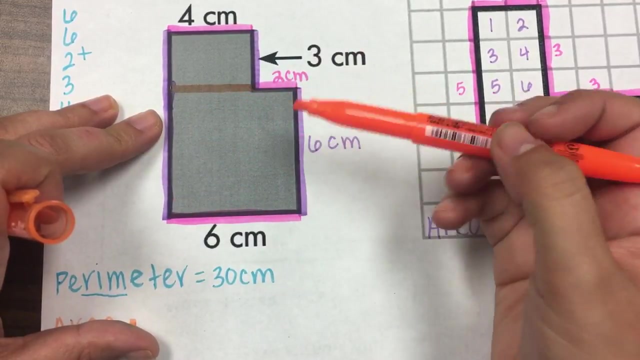 30 centimeters. okay, now to find area. Okay, To find area, we're gonna have to cut this into two pieces. so If I cut this in half Now, I have two regular shapes. I have a small rectangle up here and I have a bigger Square. and how do I know that this is a square? because this is six, and this is six and squares have equal. 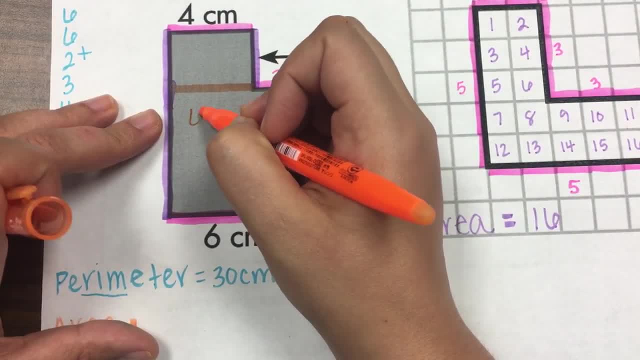 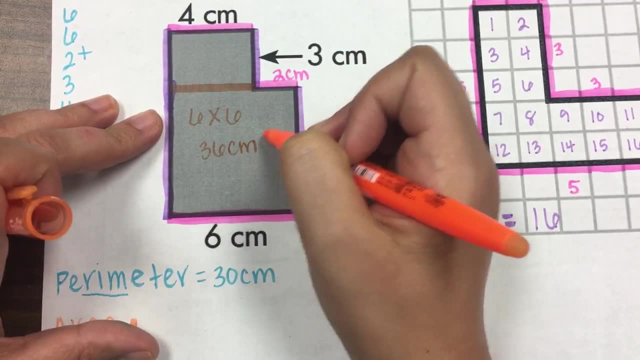 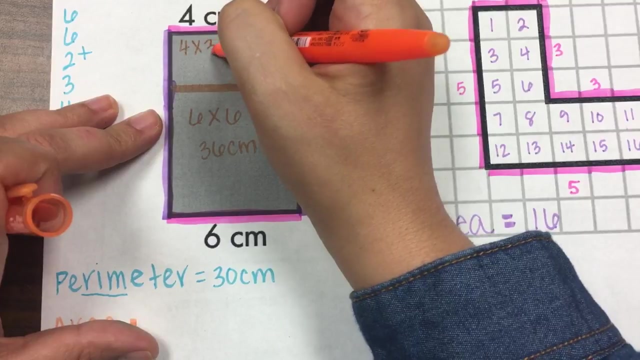 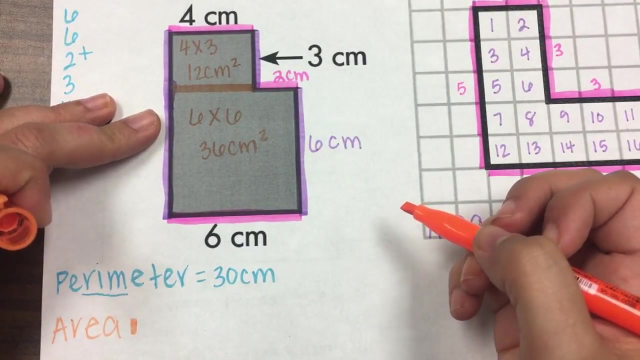 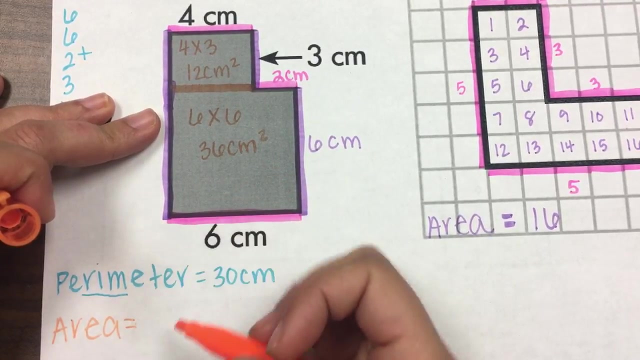 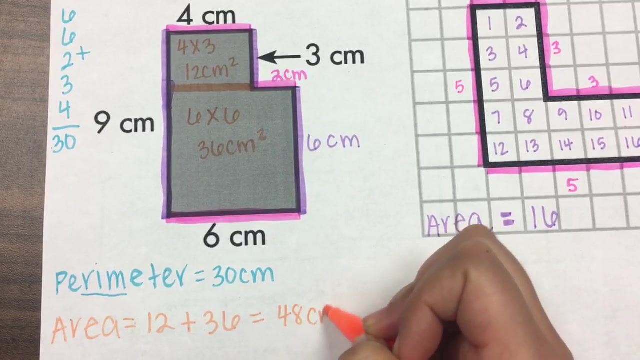 sides. So I can multiply six times six and get 36 centimeters squared, and Then up here I can multiply four times three and get 12 centimeters squared. Then I would have to combine that. So 12 plus 36 would equal 48 centimeters squared and that would be the area of the total shape. okay, 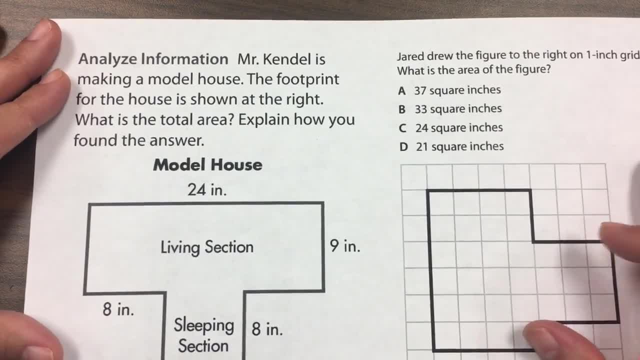 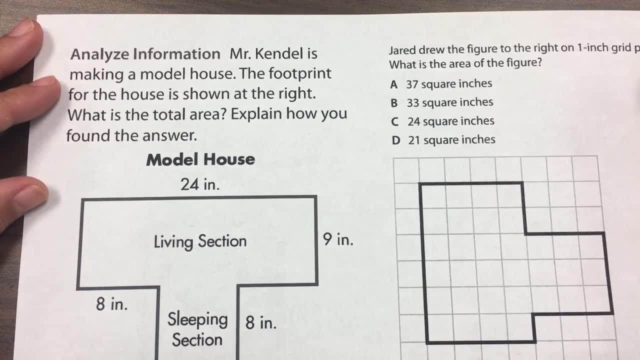 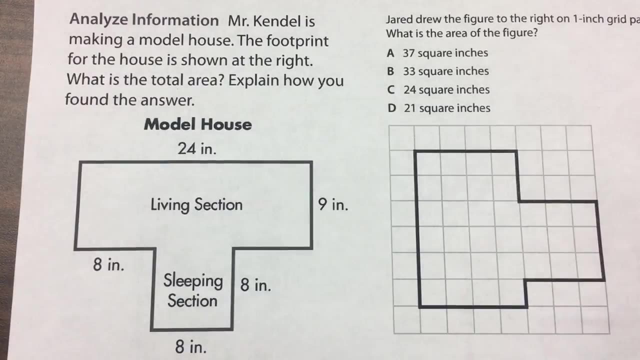 Now let's try Some word problems. Mr Kendall is making a model house. the footprint for the house is shown at the right. What is the total area? Explain your how you find your own answer. Okay. so again, we're only looking for area this time. 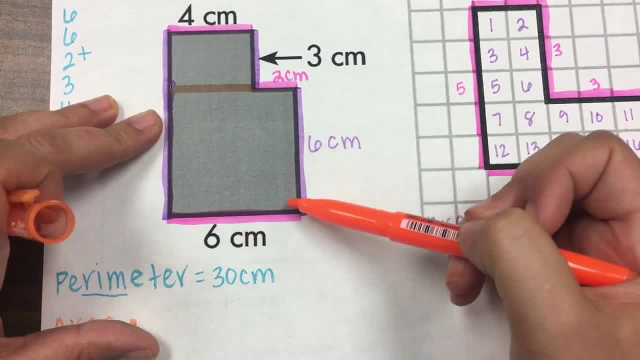 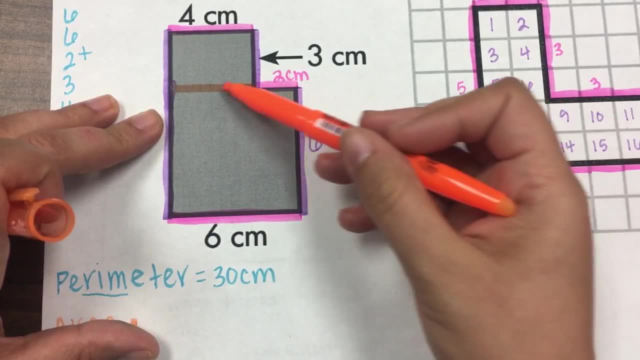 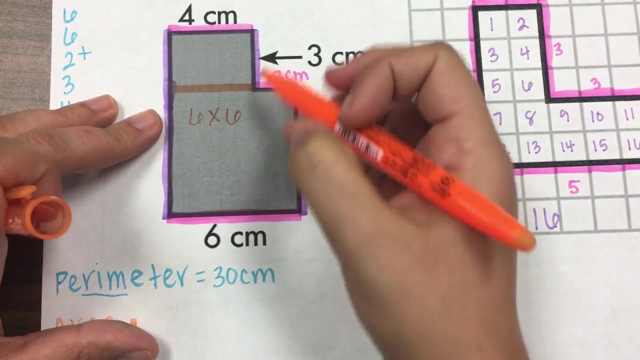 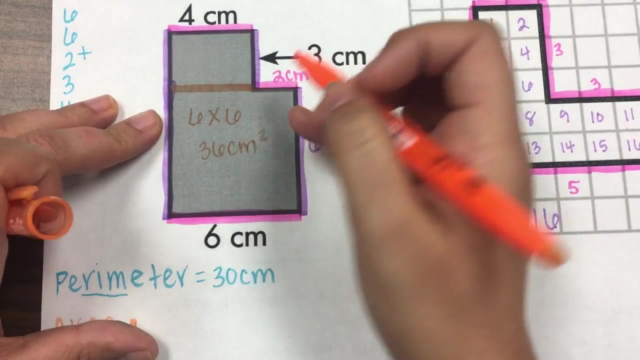 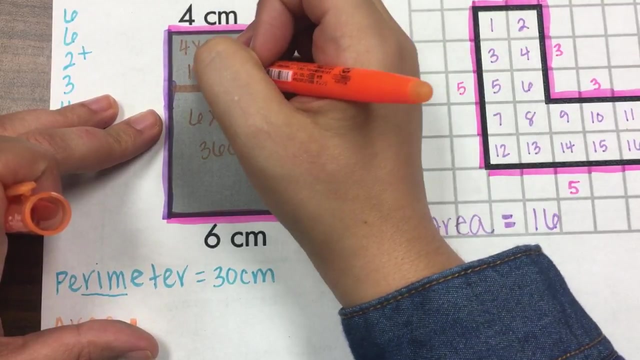 I have a bigger Square. and how do I know that this is a square? because this is six, and this is six and squares have equal sides. So I can multiply six times six and get 36 centimeters squared. and Then, up here, I can multiply four times three and get 12. 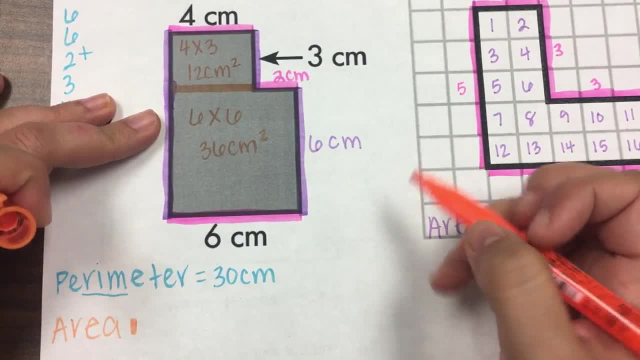 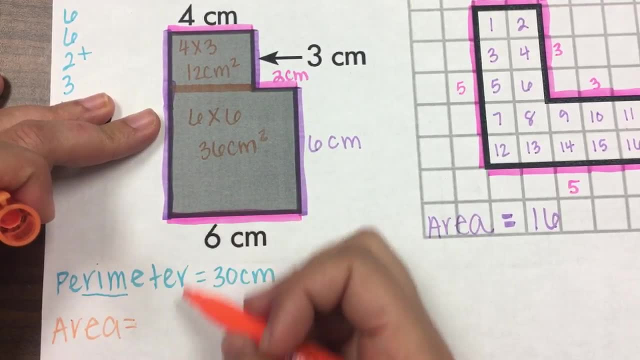 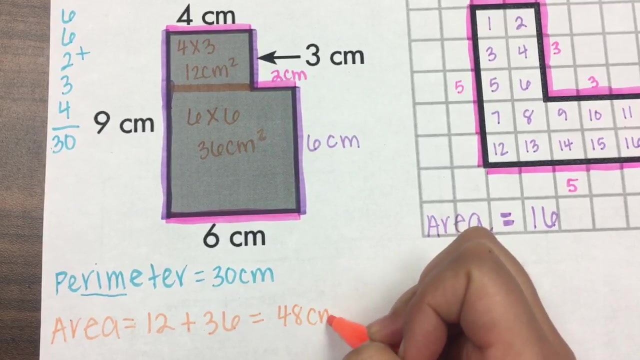 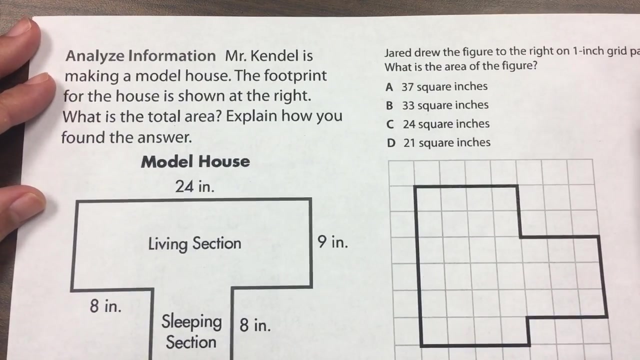 centimeters squared, Then I would have to combine that, So 12 plus 36 Would equal 48 centimeters squared, and That would be the area of the total shape. Okay, Now let's try Some word problems. Mr Kendall is making a model house. the footprint for the house is shown at the right. What is the total area? 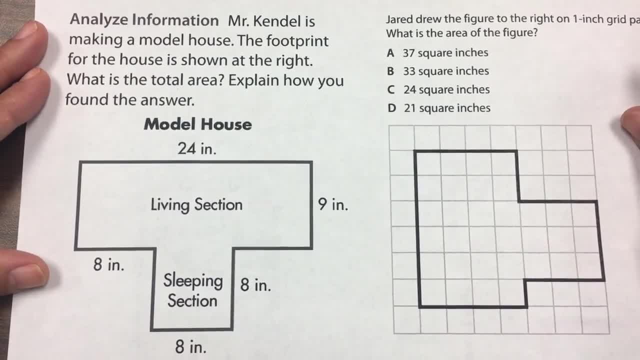 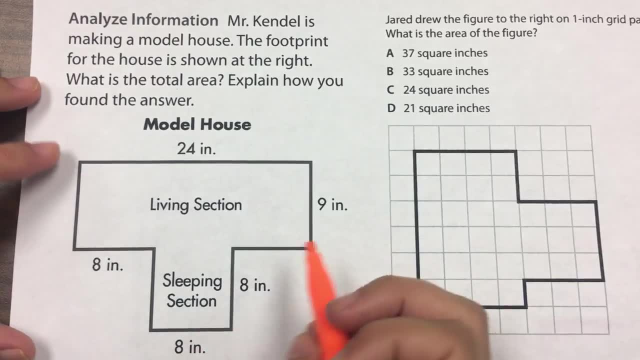 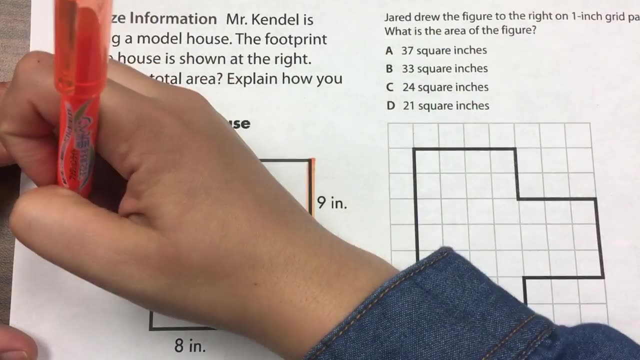 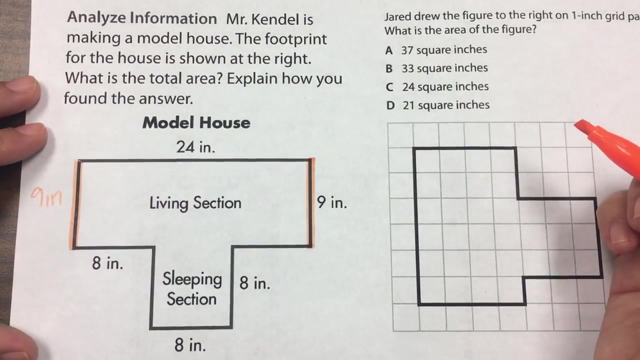 explain your how you find your answer okay. so again, we're only looking for area this time. so first I need to fill in the numbers that are missing. so if this is 9 on this side, then this also has to be 9 on the opposite side, okay, 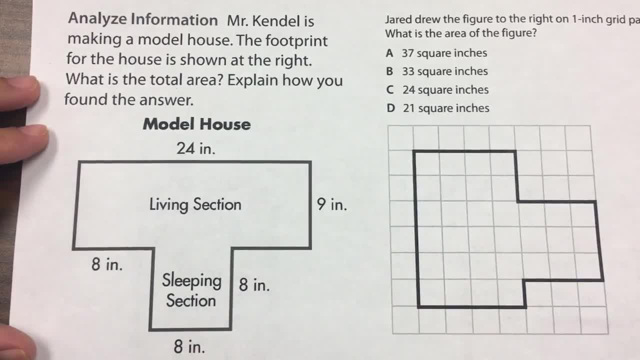 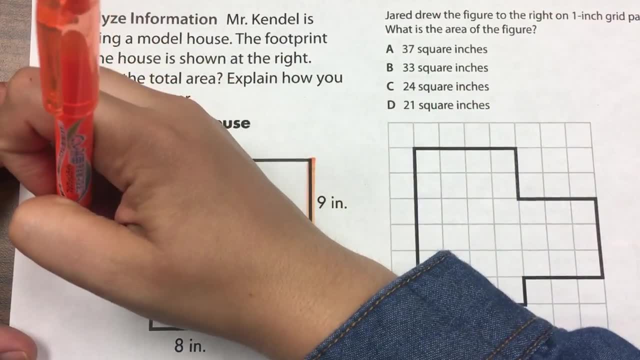 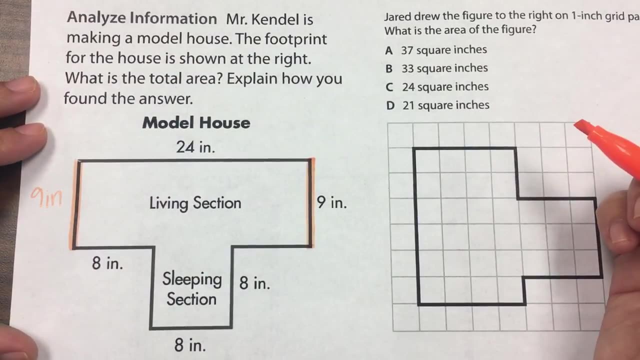 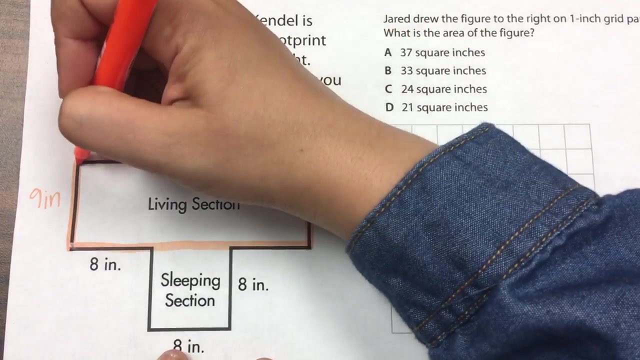 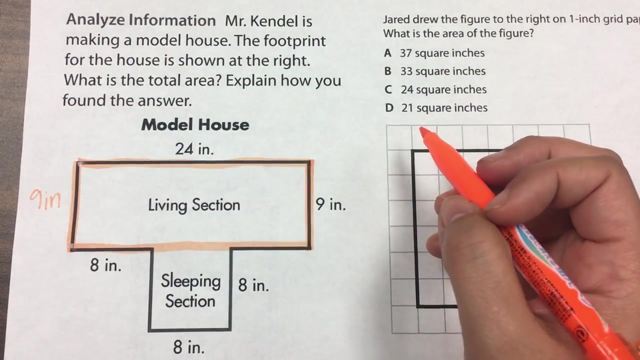 So first I need to fill in the numbers that are missing. So if this is nine on this side, Then this also has to be nine on the opposite side. Okay, now I'm going to section off This rectangle here. Okay, that's one rectangle. now I'm going to be able to multiply. 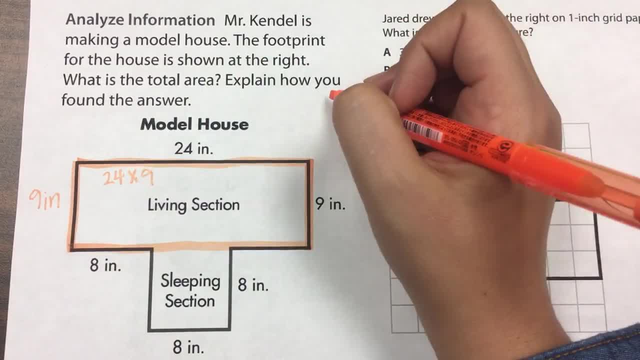 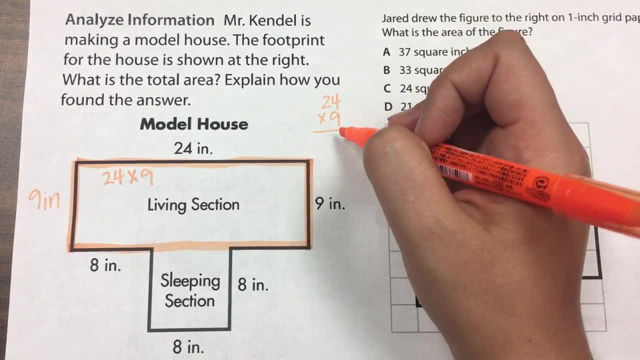 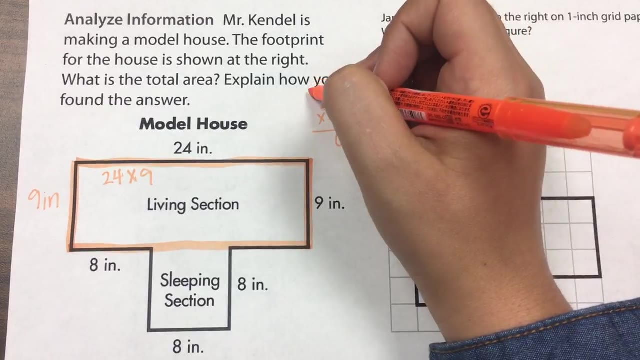 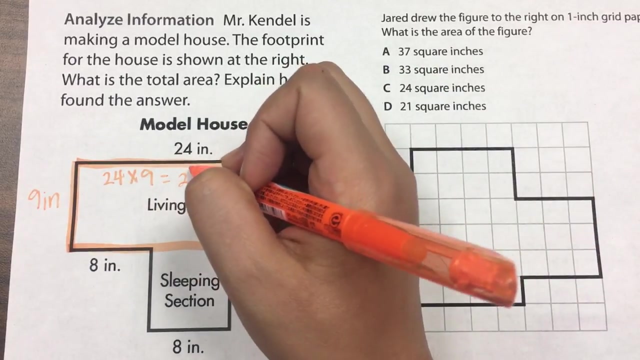 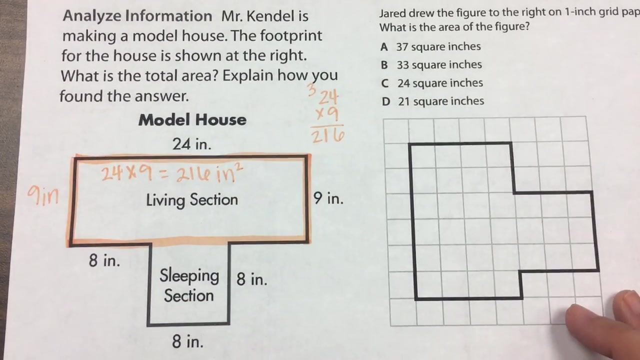 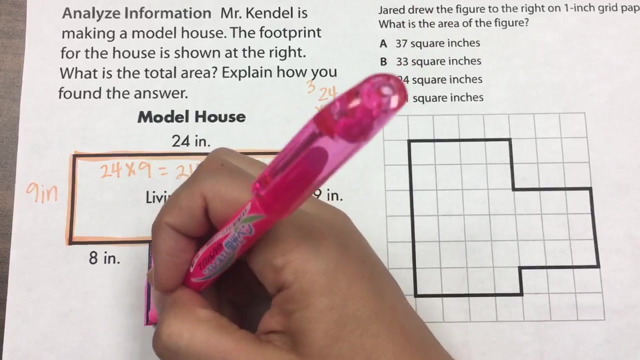 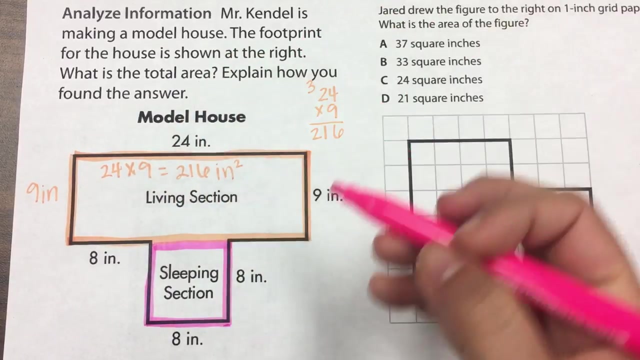 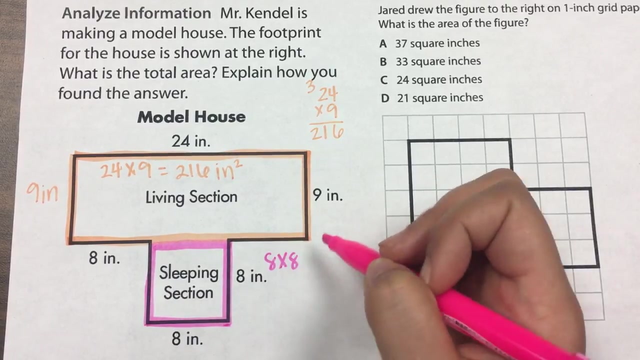 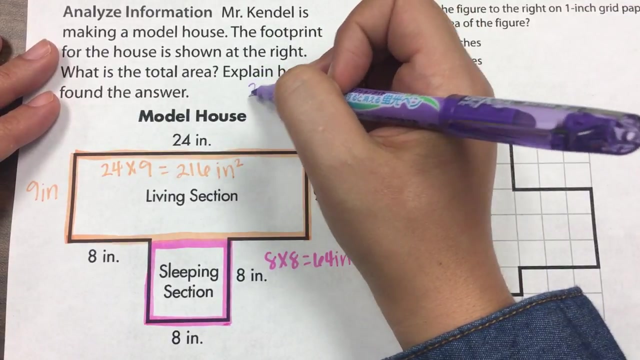 24 times nine. so nine times four Is 36, That's 18- 21. Okay, now I'm going to do the square down here at the bottom, okay, so here we have to multiply 8 times 8 is 64 inches squared, and finally we add 216 plus 64. 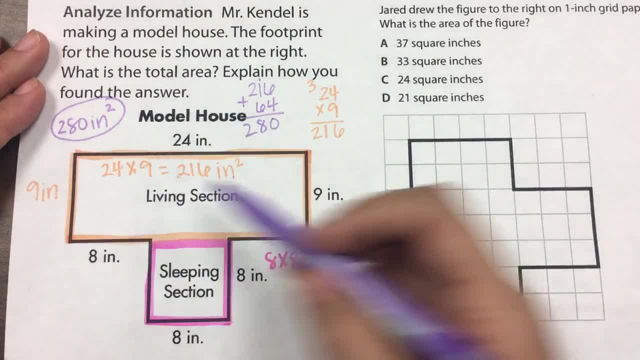 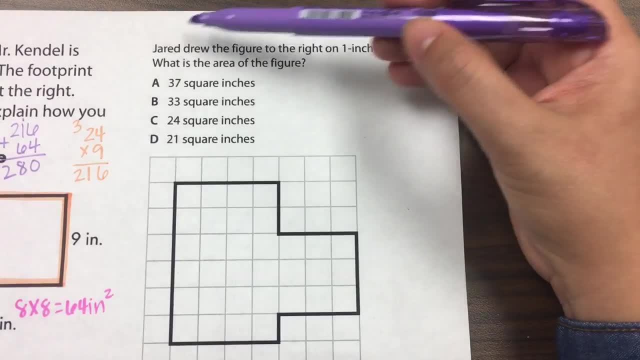 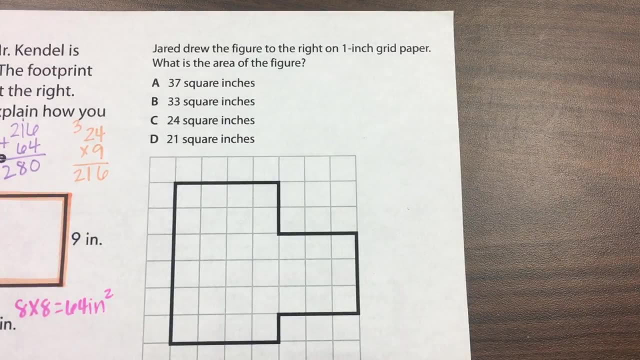 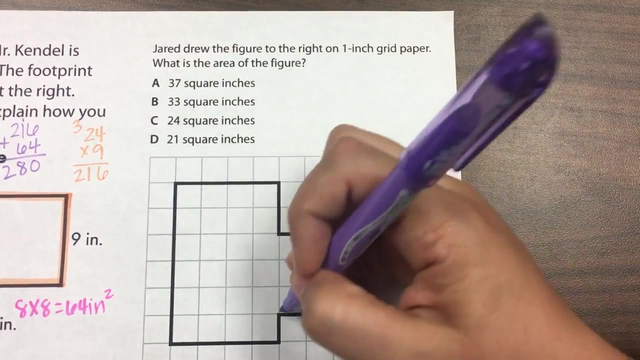 and this would be the total area of the entire house. for the next one says: Jared drew the figure to the right on one inch grid paper. what is the area of the figure? okay, for this one it's a little bit easier because we're able to section off two separate. 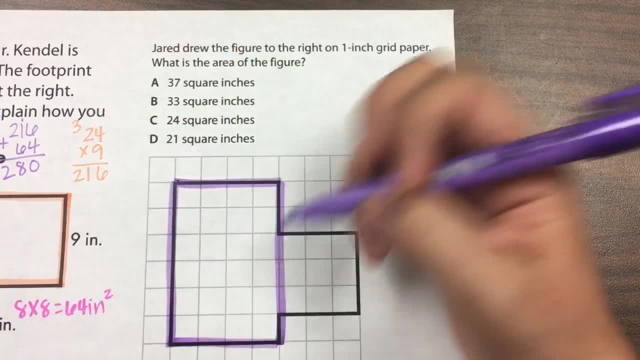 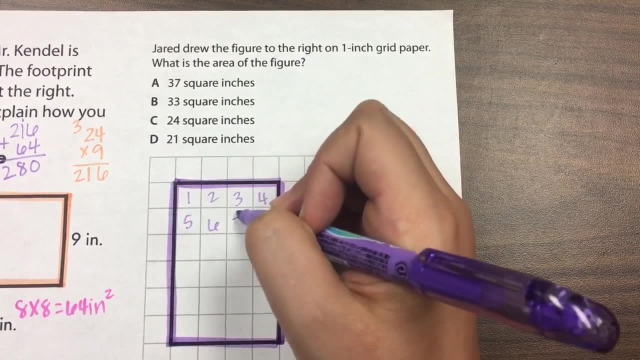 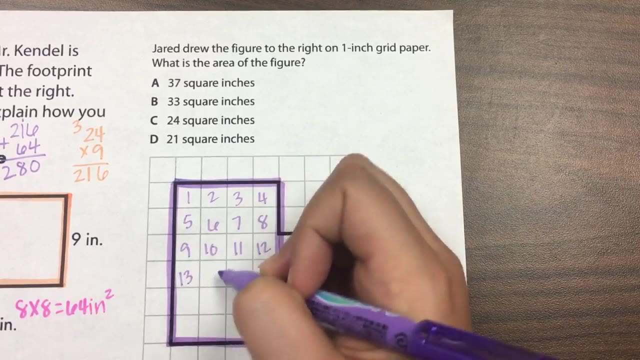 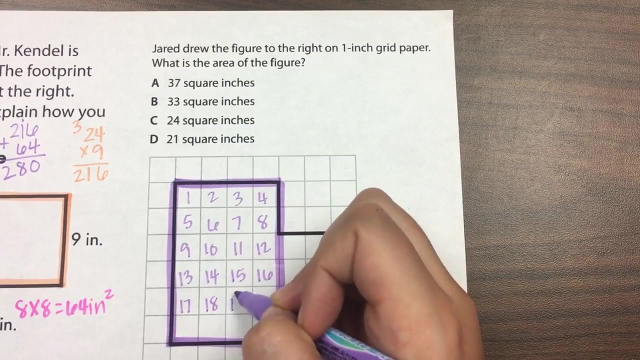 pieces. okay, now I'm going to count this one: 1, 2, 3, 4, 5, 6, 7, 8, 9, 10, 11, 12, 13, 14, 15, 16, 17, 18, 19, 20, 21, 22, 23. 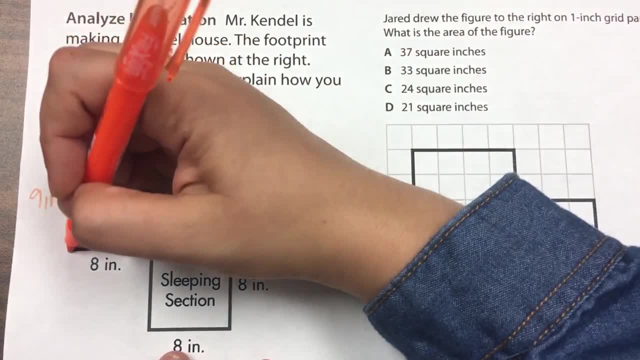 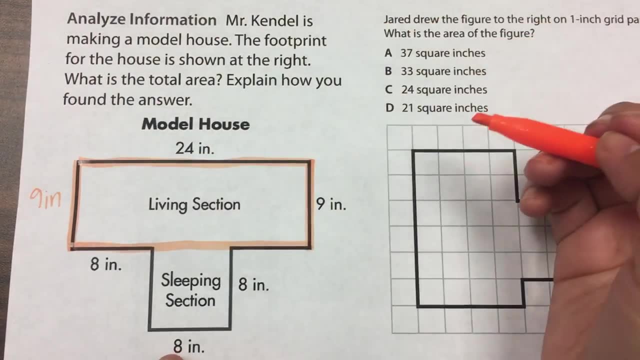 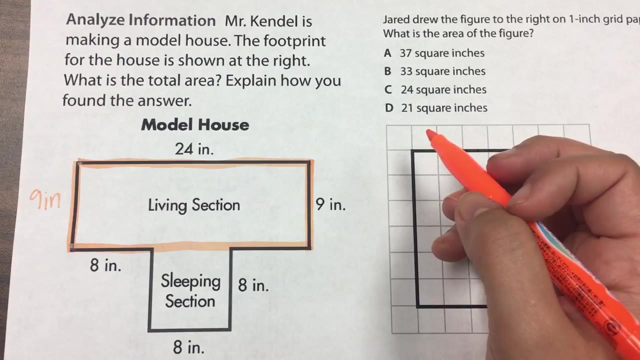 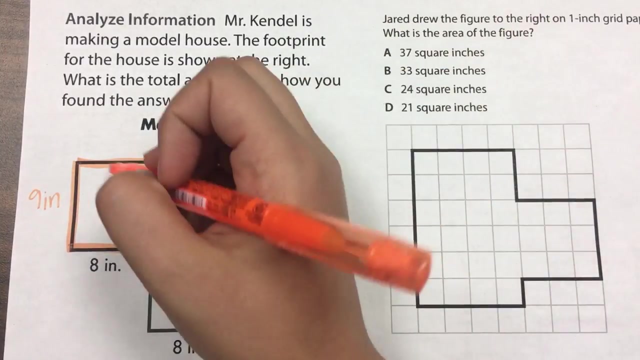 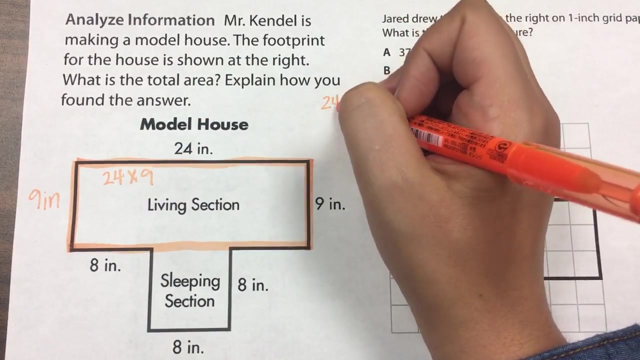 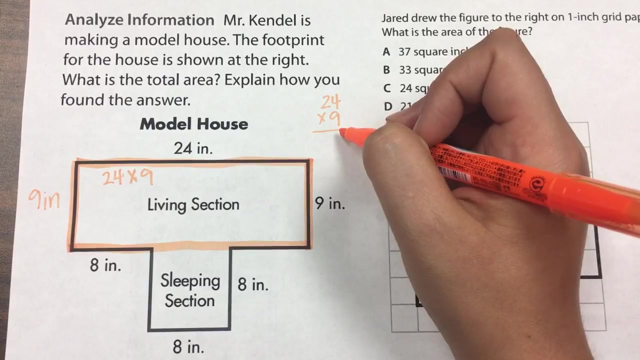 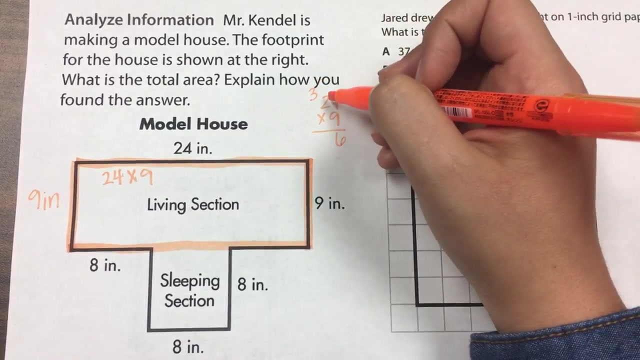 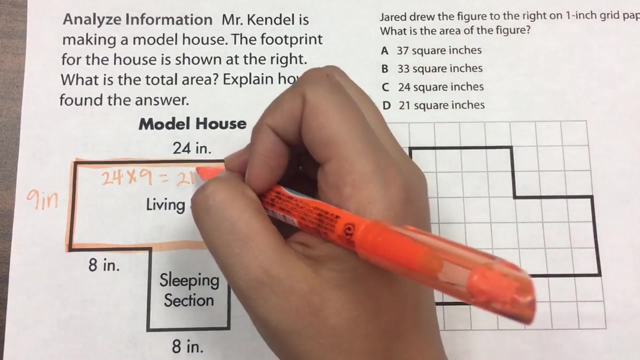 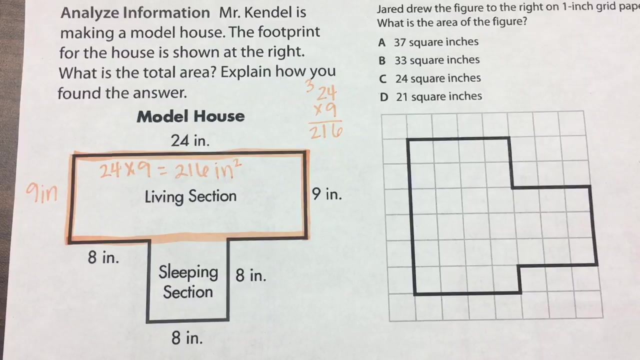 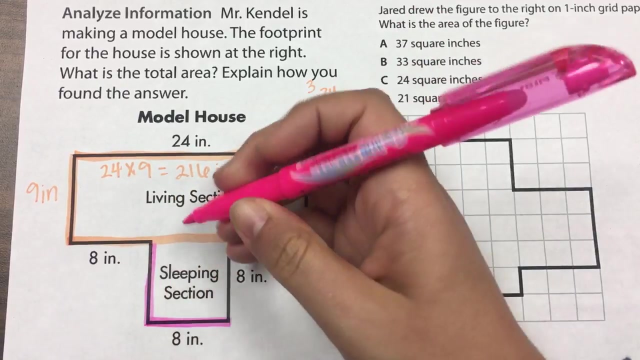 now I'm going to section off this rectangle here. okay, that's one rectangle. now I'm going to be able to multiply 24 times 9. so 9 times 4 is 36, that's 18 and 21. okay, now we're going to do the square down here at the bottom. 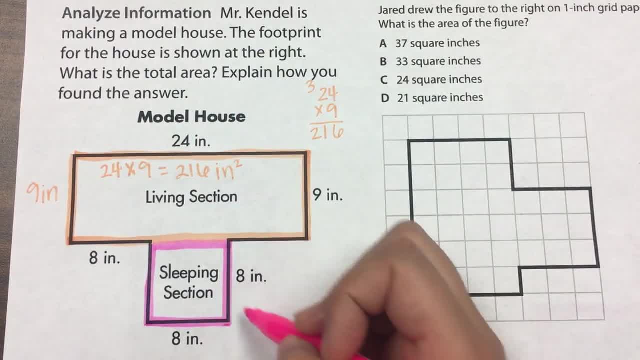 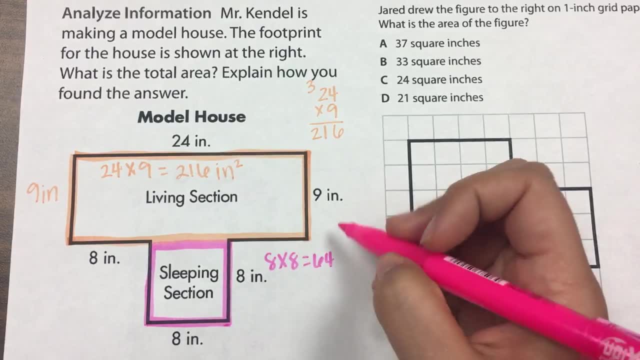 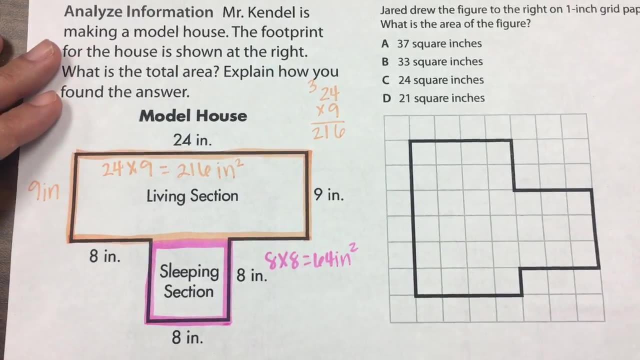 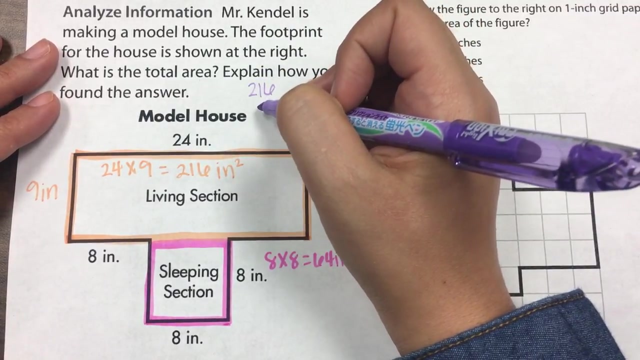 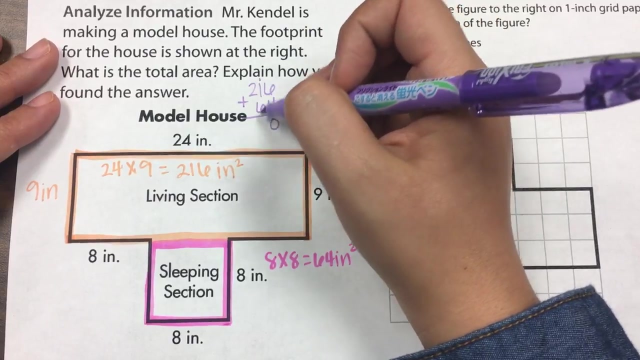 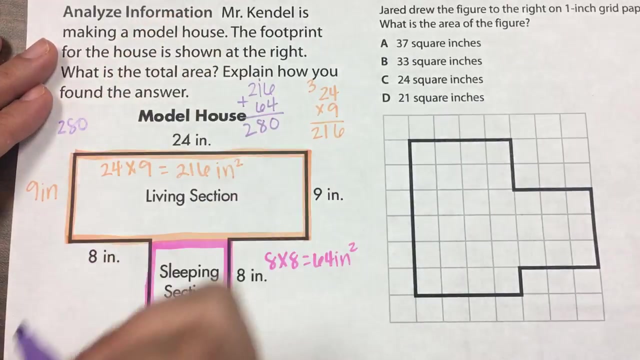 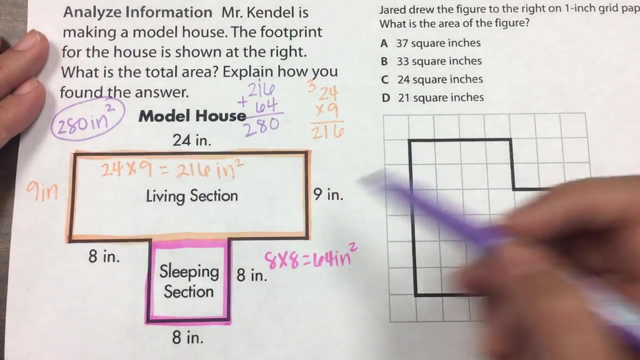 okay, so here we have to multiply 8 times 8 is 64 inches squared, and finally we add 216 plus 64, 216 plus 64, and this would be the total area of the entire house, and this would be the total area of the entire house. 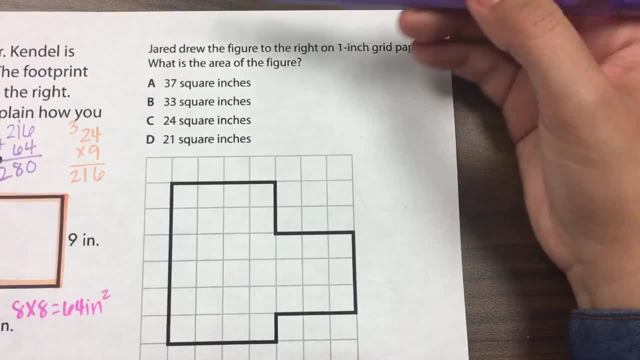 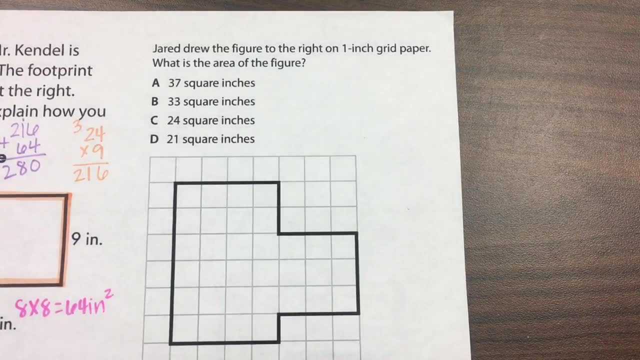 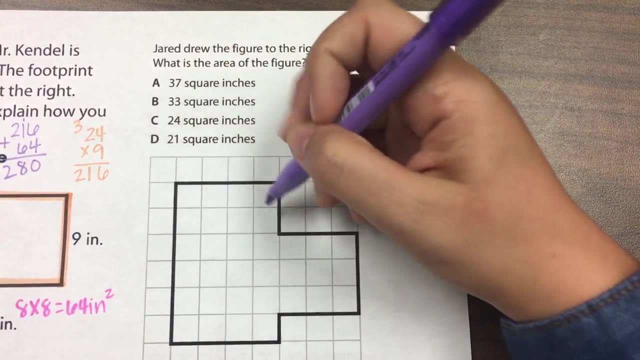 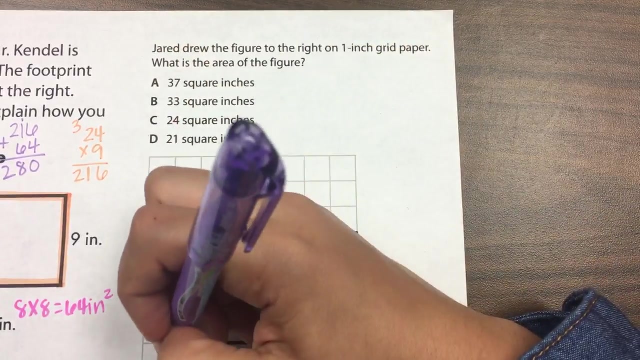 For the next one, it says: Jared drew the figure to the right on 1-inch grid paper. What is the area of the figure? Okay, for this one it's a little bit easier because we're able to section off two separate pieces. 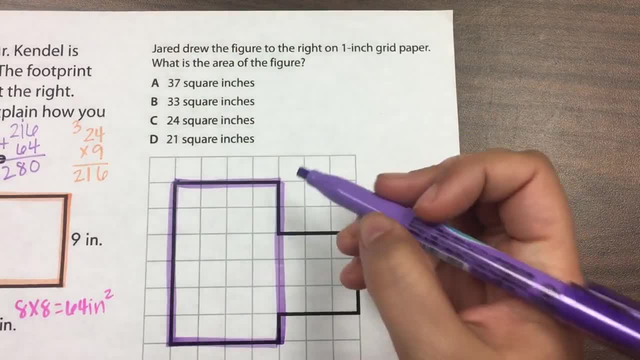 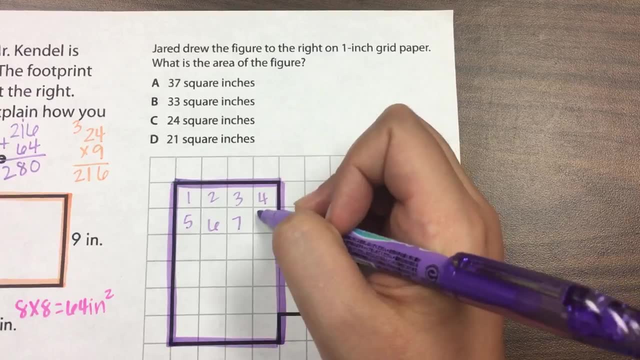 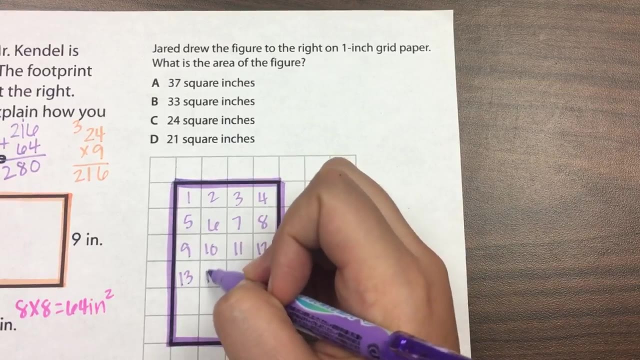 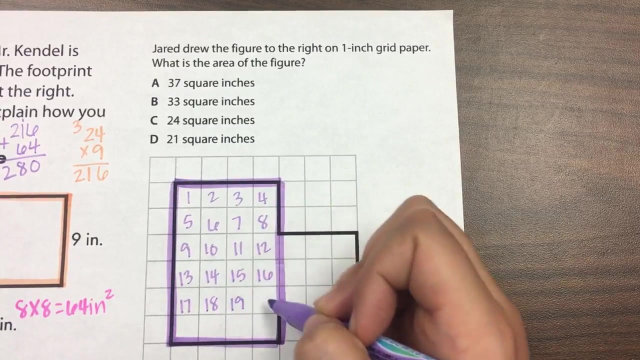 Okay, now I'm going to count this one: 1,, 2,, 3,, 4,, 5,, 6,, 7,, 8,, 9,, 10,, 11,, 12,, 13,, 14,, 15,, 16,, 17,, 18,, 19,, 20,, 21,, 22,, 23,, 24,, 25,, 26,, 27,, 28,, 29,, 30. 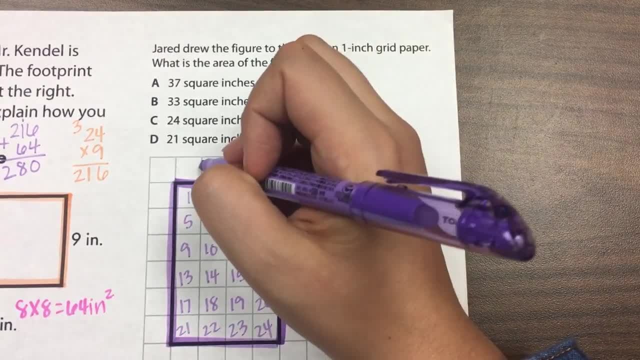 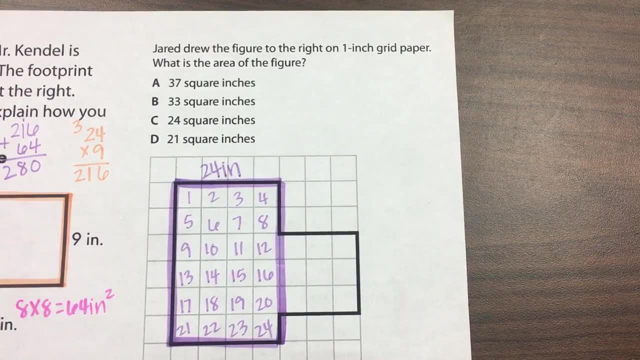 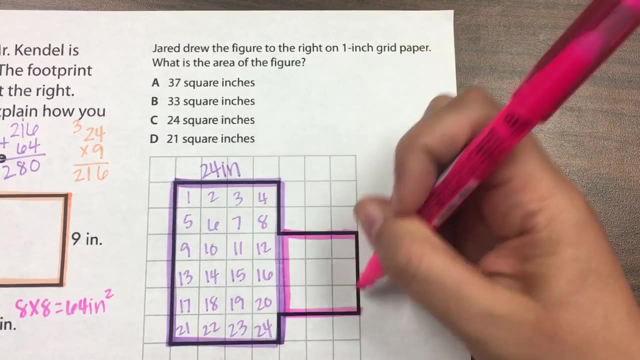 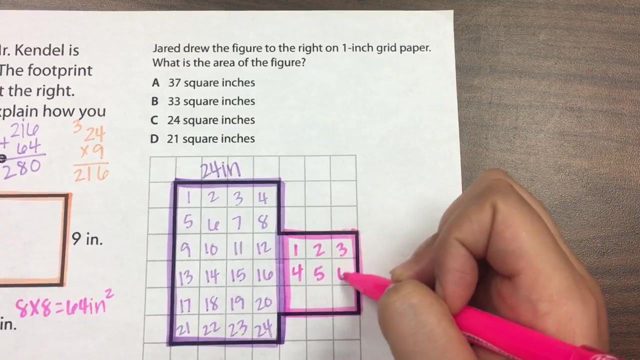 23 and 24.. So I have 24 inches here. Now let's try the other side, This right here: Don't forget about this one. We have 1, 2,, 3,, 4,, 5,, 6,, 7,, 8,, 9.. 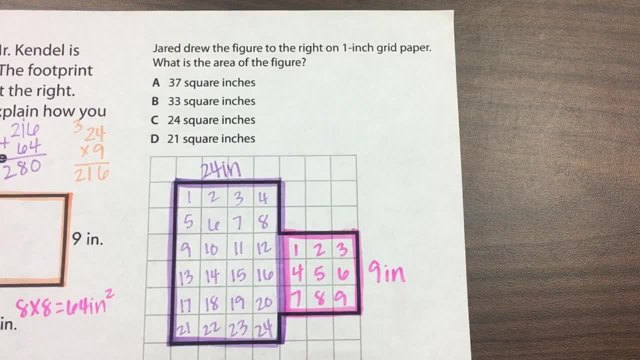 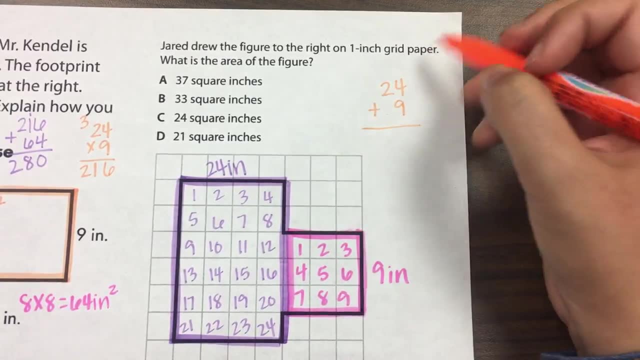 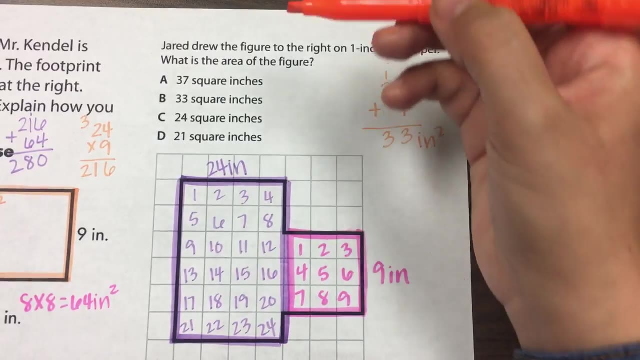 So this is 9 inches And finally we add 24 plus 9 is 33 inches squared. That's it.